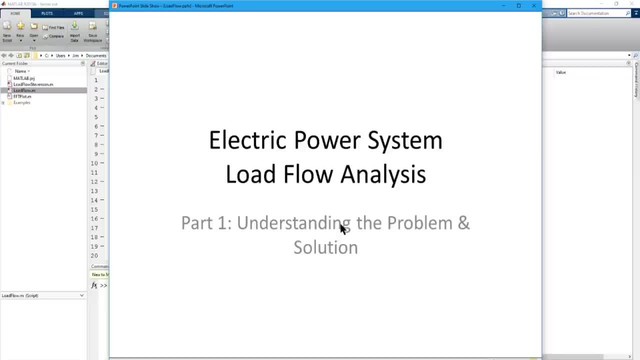 to solve the problem. So then the equations make a whole lot more sense. And then you can jump into the equation, Say, oh yeah, now I know what they're doing. So we're going to start out here with a very 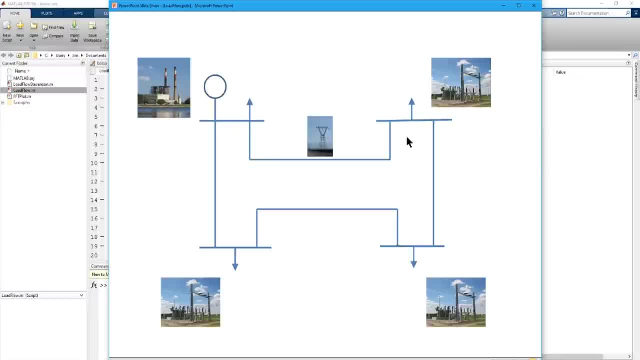 very simple electric power system And you can see I've got four buses. These horizontal lines are buses, And up in the top left I've got a bus with a generator connected. And that's what this circle is. And you can see here a photograph of a generating station And each arrow in each. 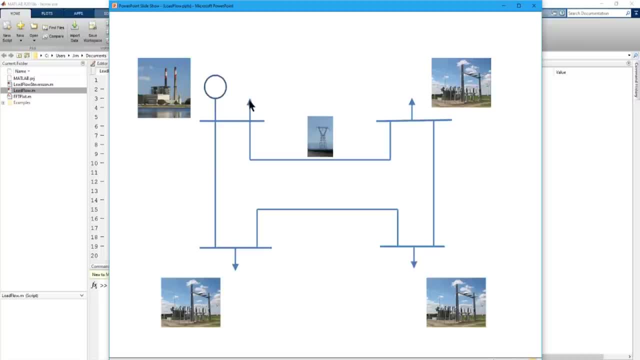 of these buses represents a load, watts and vars being consumed at that bus. So the power station, you've got load for all the auxiliary equipment And these other buses. I've basically got just power consumption by customers, which is distribution or sub-transmission substations, And you can see the photographs here And these: 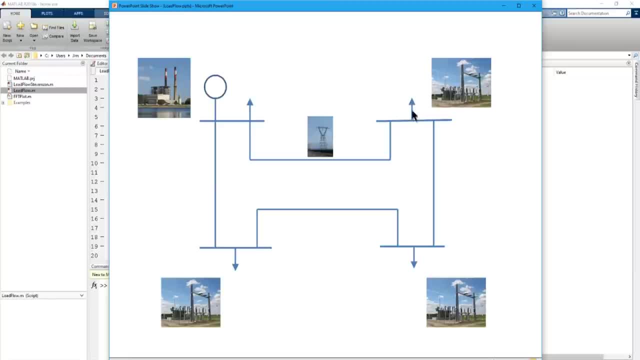 arrows again are the megawatts or watts and vars being consumed at these substations And tying all of these four buses together. these substations are transmission lines. I've got a photograph here of a transmission line And I've got one, two, three, four transmission lines tying these buses together in a network. 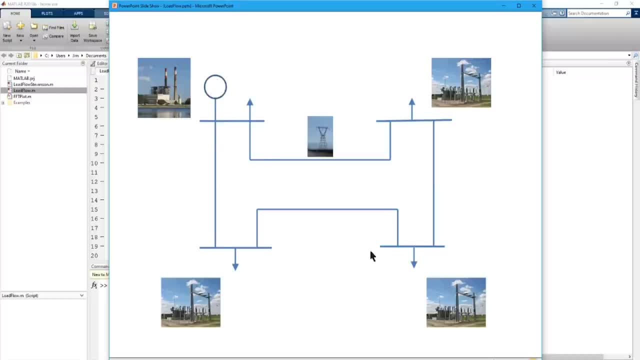 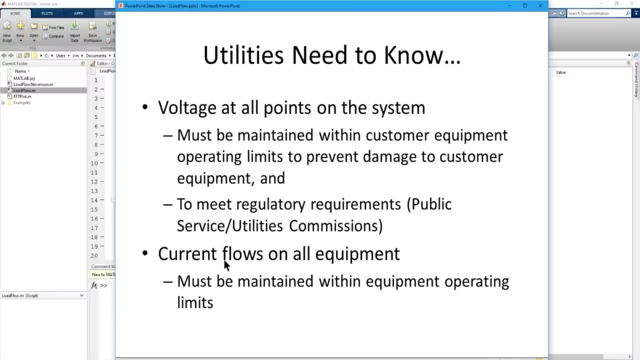 And the generating station generates power And it flows to these substations where the load is, And it serves the load through these transmission lines. So utilities need to know a couple things, And that's what we're going to be addressing in this problem and solution. 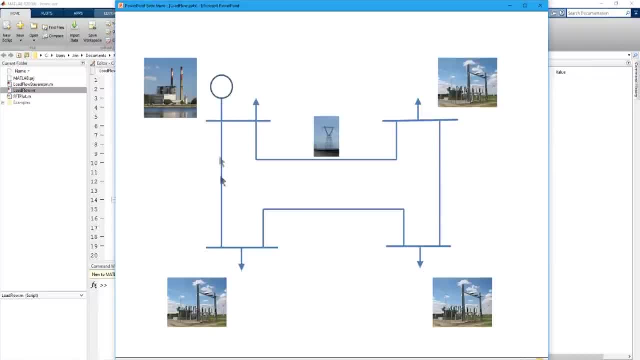 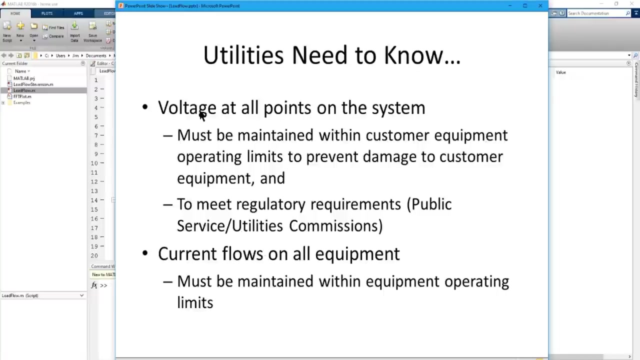 Utilities need to know on this power system that they've got, and generally most utilities have nothing like this very simple system. In fact, they have hundreds or thousands of substations and transmission lines and power plants all tied together in a very complicated power system And there are a couple things that they need to know about their power system. One: 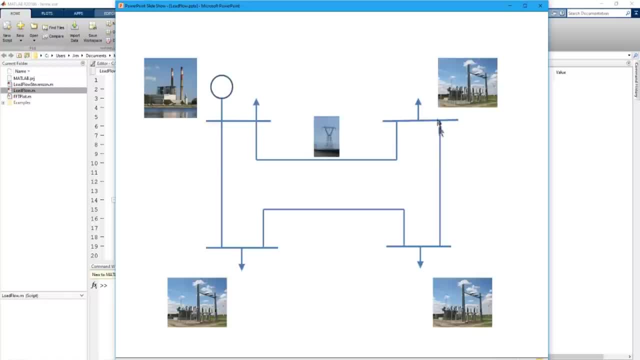 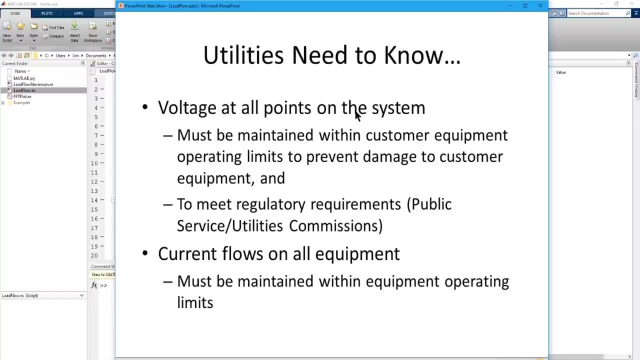 of them, one of the most important is they need to know at each point, at each of these substations. they need to know the voltage at every point on their system And generally they need to know like a worst-case voltage, In the worst case, what is the voltage going to be And why do they need to. 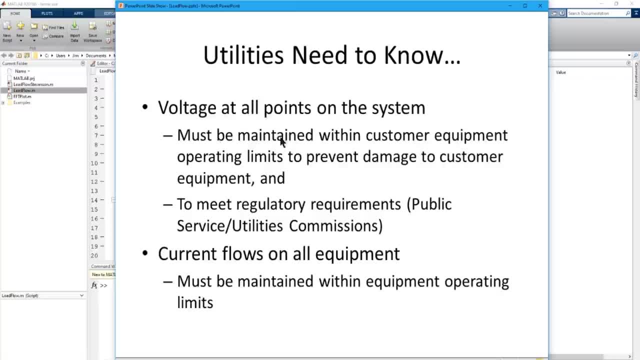 know that Well, the voltage at their substations and at their customers must be maintained within a very tight range of voltage. Why is that? Well, all of the or most of the equipment that customers, that you have in your house connected to your outlet that's fed by the electric utility. 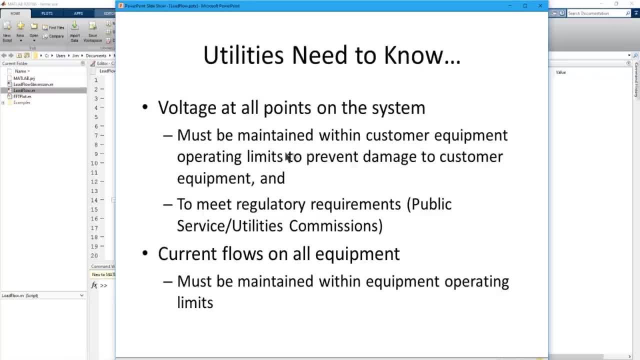 the voltage on that equipment generally needs to be maintained within a very small range, a very tight range of voltage. And the reason that that's the case is because if it, if it strays too far out of that range of voltage, it can cause damage to the equipment. 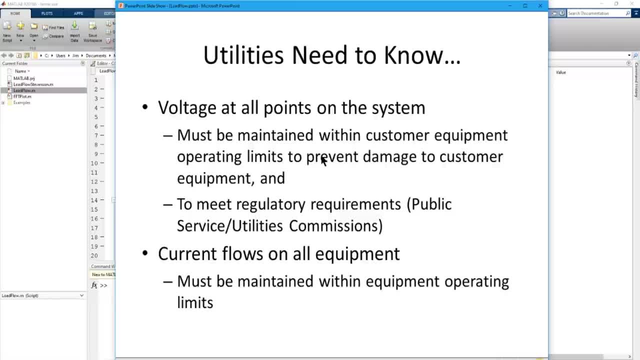 For example, your air conditioner, your refrigerator. those types of equipment can only be run in a narrow range of voltage. If you don't, for example if your refrigerator, if the voltage is too low, the refrigerator won't cool and it could cause damage to the motor. if 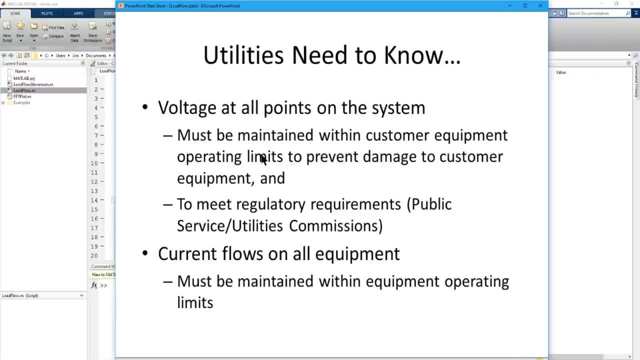 it's low enough. So it's important to maintain voltage in very strict limits at the customer and at the substations, And generally that can be within something like plus or minus five percent, or maybe ten percent in some cases. So it's got to be a very narrow. 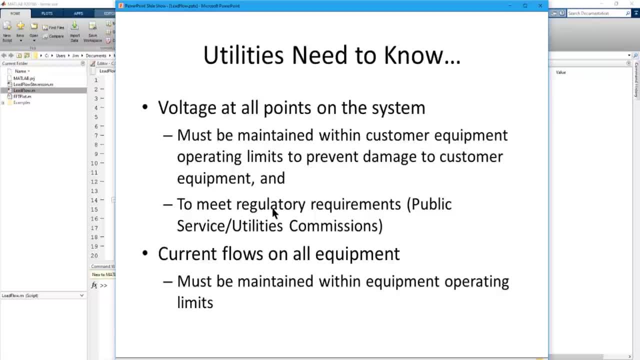 range of voltage. And since that's so important, the government regulatory commissions, like the public service or utilities commissions in each state have strict requirements for the utilities that they maintain their voltage in a very narrow range. So voltage is very important, So utilities need to know at all points on their system what the voltage is going to be. generally, 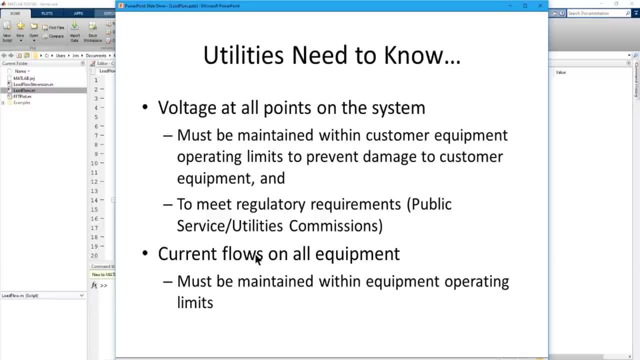 in the worst case scenario- And also current. They need to know what current is flowing on all their equipment, their transmission lines and their substations, because that current also has to be maintained within a range that the equipment can handle. If it's outside that range, 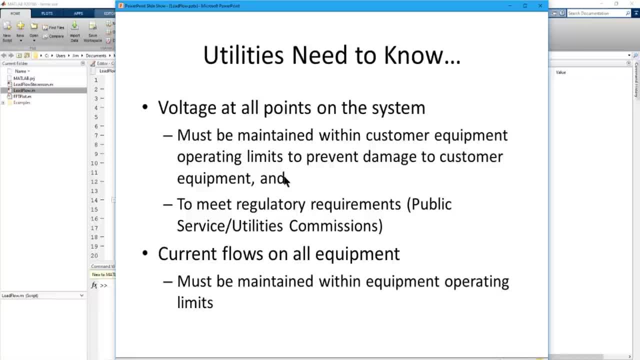 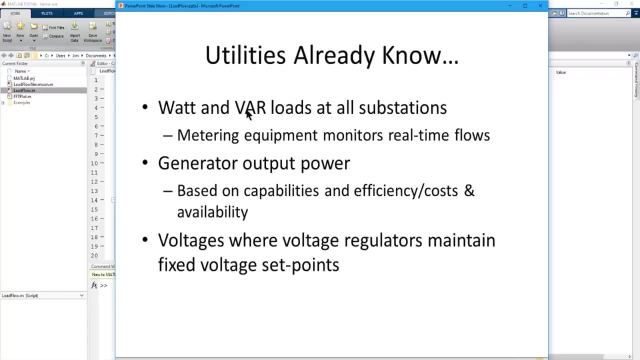 you might overheat the equipment or cause damage. So utilities need to know generally the voltage on their system and also the current flowing on their equipment. Now they already know some things that can help them figure out what the voltage is and what the currents are. In most cases utilities know at all of their 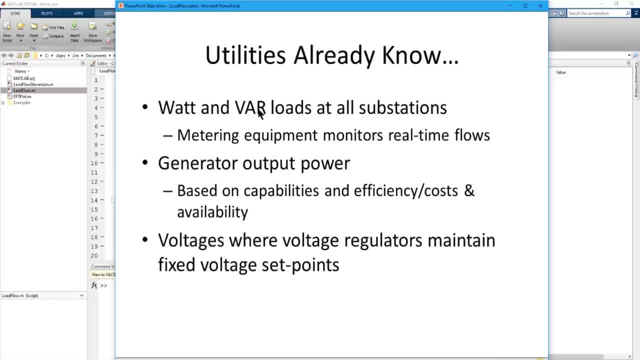 substations what the watts and VAR loads are on all of the circuits going out to the customers. Most utilities, most of their substations, have equipment monitoring the watts and VARs flowing on their circuits going out to their customers, often in real time or at least historical. 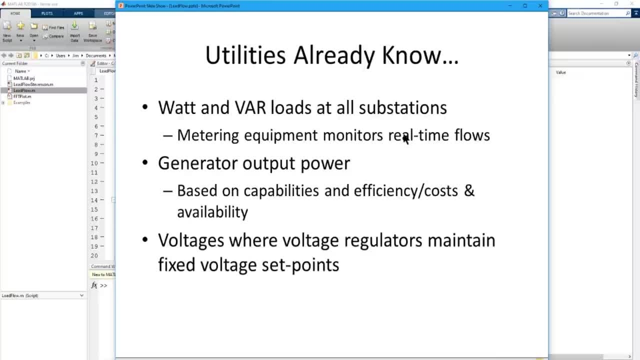 manually recorded. So they have really good information about worst case and real-time watts and VAR flows at their substations. They also know generally what the output power of each of their generators is. They know the ratings. They buy like a 100 megawatt generator. They know the capabilities. 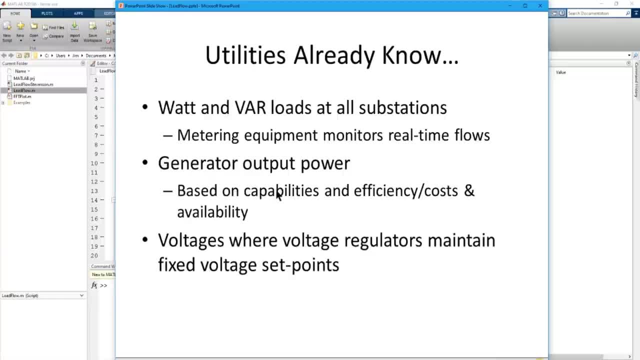 what it's rated to, what power output it's rated at. But also they know, for example, each generator has a certain cost of fuel and operation to run that generator And they know which generators are more cost effective to run and which are. 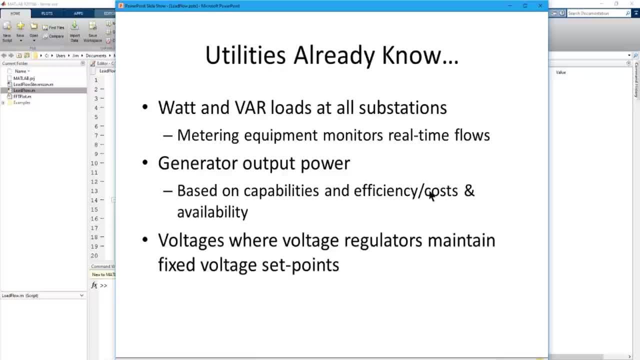 least cost effective to run. So they know, based on the costs and also the availability, if that generator is available or when it's available, they know what the output power is going to be. because, for example, If it's a very cost effective and relatively low cost to run that unit, for example if it's a nuclear plant, they generally want to run the low cost, like a nuclear plant, 24-7 at maximum power, because it's the cheapest generation source compared to another that might cost more. 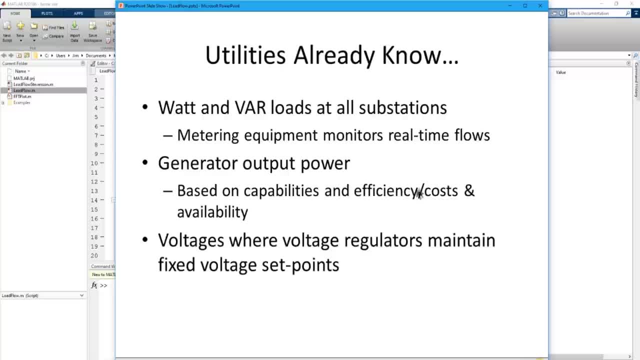 Maybe a wind generator might cost more, so they might not run that as much and it might not be available as much if the wind's not blowing. So generally they can manage what the output of their generator is going to be. They know what it's going to be, So output power of generators is something they generally have a pretty good idea of what that will be. 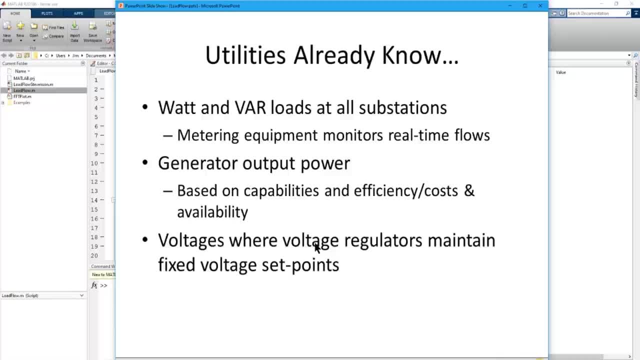 And the third thing: in some cases, especially where there are generators at the At the bus, they know what the voltage is going to be because each generator generally has what's called a voltage regulator that can be set to maintain a fixed voltage at that substation bus. 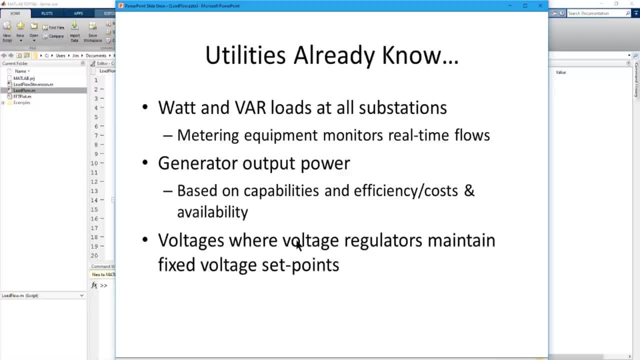 So they might set it at, for example, 1.02 per unit and the generator will continually maintain that voltage. At most buses this doesn't exist, but at some buses, like generating buses or buses where voltage Regulators on other equipment are installed, they have a pretty good idea of what the voltage is. 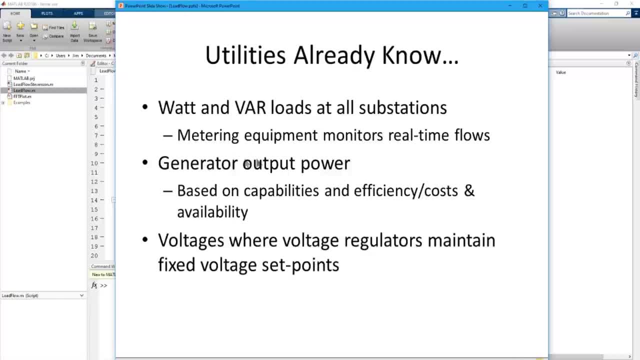 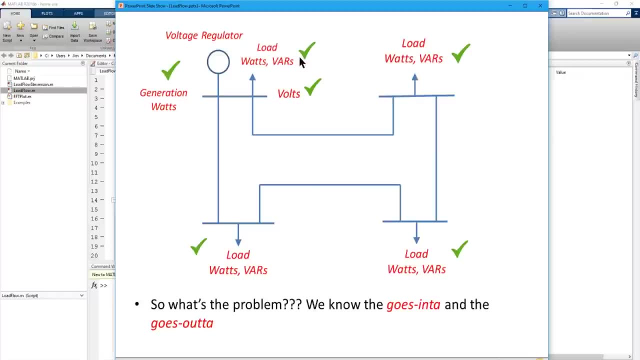 So there are some things- watts and VAR loads, generator output power and voltages at some buses- that the utilities know. that can help them figure out what they don't know. So here's our system and I've made a note of those things that the utilities generally know about their system. 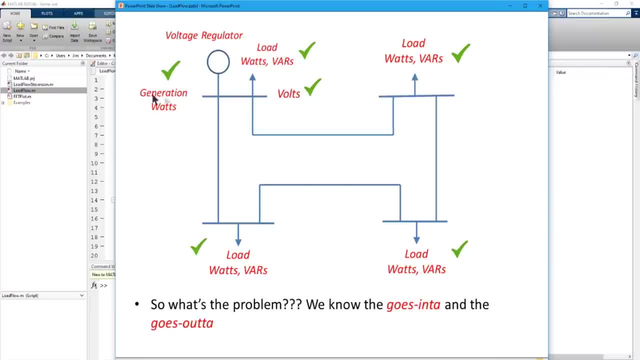 They know here's a generator. They know how much Output power this generator is going to be providing. They know whatever load in watts and VARs might be consumed at this generator bus. And this is a, Since it's a generation source with a voltage regulator. they know the voltage here. 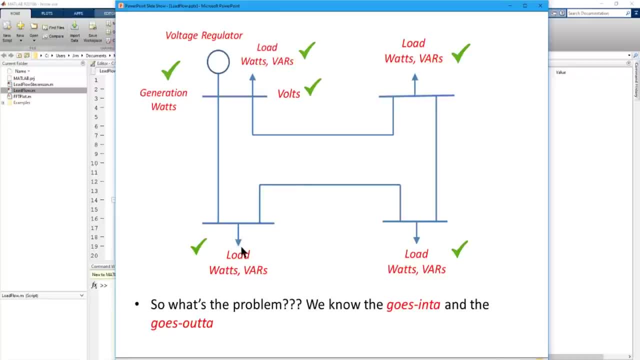 At these other buses, which are basically just load buses, no generation. they know watts and VARs at each of these. So this is basically what the utility knows. So you might look at this And say, well, wait a minute. 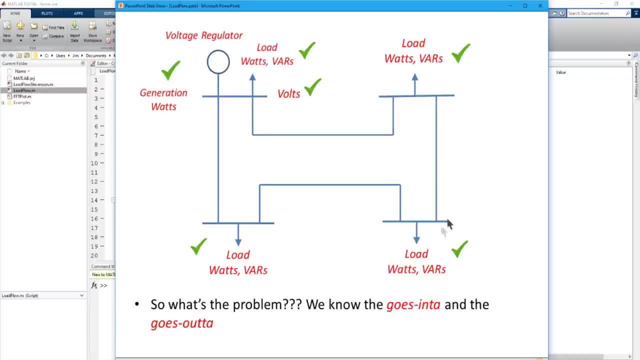 They know the voltage here, They know the load at each of the stations And they know what the output power of the generators is. So what's the problem? They know what's going into the network And they know what's coming out. 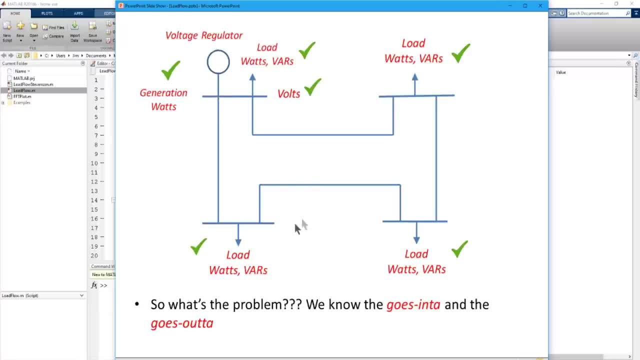 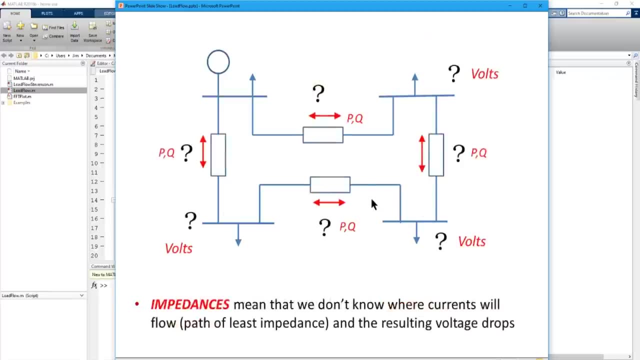 Just add these up. And if it's the same as the generation, then why is there a question? They know, We know the goes into And we know the goes out of. So what's the question? Well, what we haven't mentioned yet is impedance. 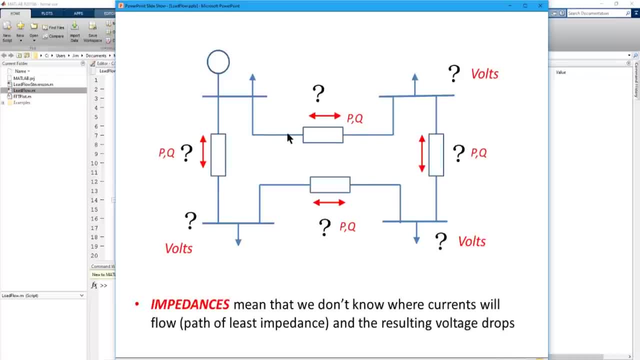 So what's the question? Well, what we haven't mentioned yet is impedance, And each of these transmission lines connecting each bus has an impedance that can be easily calculated, And in fact it's about half an ohm, or something like that, per mile of transmission line. 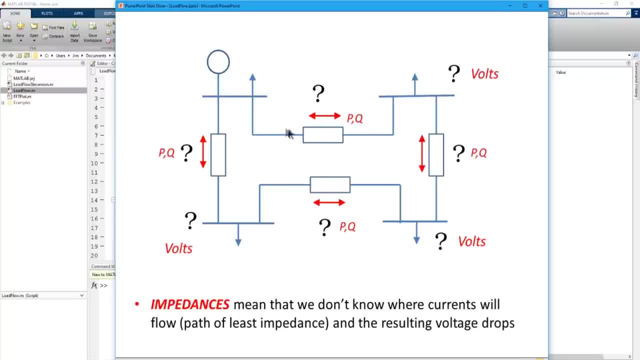 And these impedances. the existence of these impedances means that, as current flows in this network, the current will generally choose the path of least impedance Right. So how it flows, based on the load, Based on the loads at these buses and the generation these flows on these lines, can change. 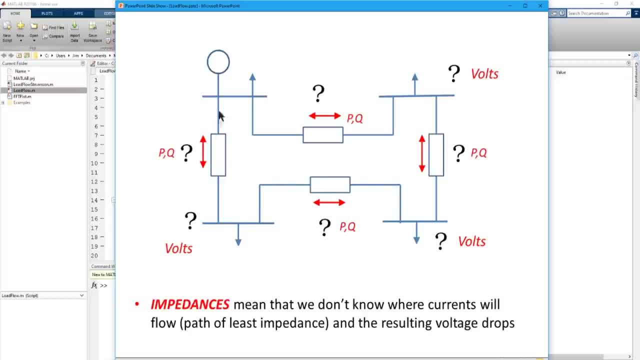 And as the flows change, that means the voltage drop across. these impedances change, which means the resulting bus voltages at these load stations changes. So the flows and the resulting bus voltages is a big question mark. We don't know. It depends on the loads here and the relative impedances of the line. 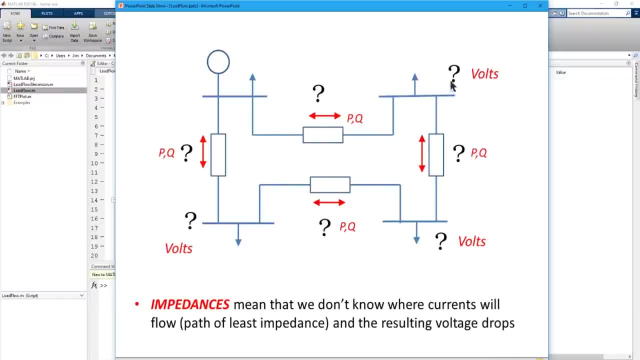 So they need to calculate the flows and the voltage based on these impedances. Now the other thing they need to consider is outages. For example, if a line comes out of service, the voltages may be lower because now you have load flowing on this line going all the way around the loop here to get to the station. 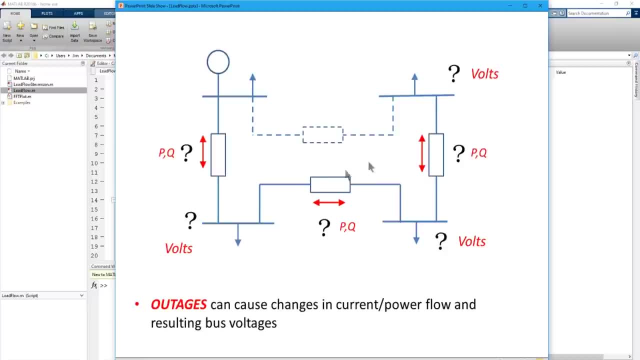 So the voltage drop might be more. So utilities need to calculate, with a given network of these impedances, How the inputs and outputs, how they're going to flow through the network, based on the configuration of the system and the impedances, and which elements of the system are in service or out of service. 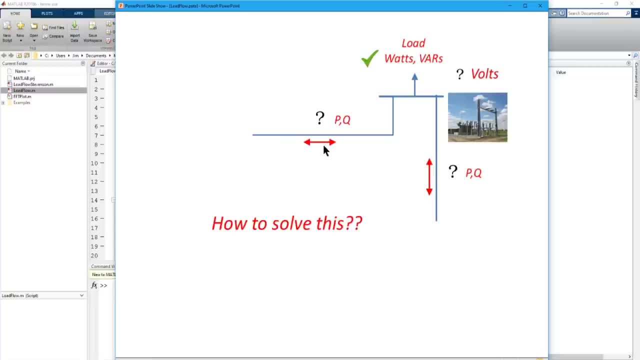 So we have a lot of unknowns and we have some things that we know. So let's look at a very simple look at just one bus in the system- a load bus, a substation bus- And let's figure it out. Well, how are we going to know? 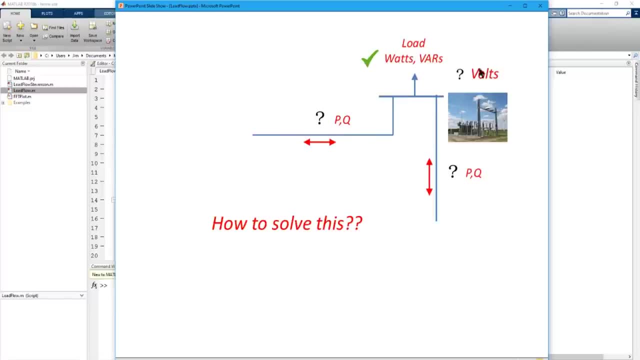 How are we going to solve this? I mean, we don't know the voltage at this bus. If we want to solve this voltage for this bus here, we don't know the voltage, We don't know the flows on the line, So we're not going to be able to figure out the voltage drop, to figure out what the ultimate voltage here. 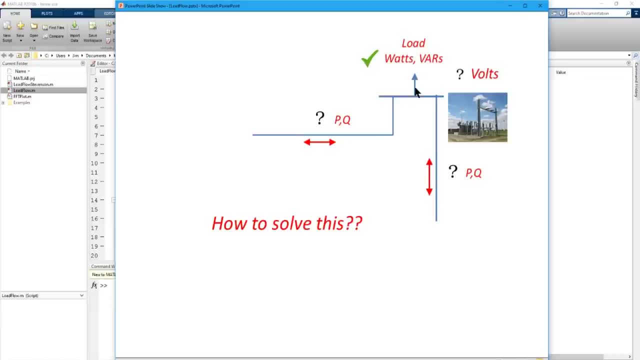 All we know is the watts and VARs being consumed or sent out to customers at this substation. So how are we going to solve this for voltage and how are we going to figure out the flows? Well, let's step back and see. what do we know about the system that might help us figure this out? 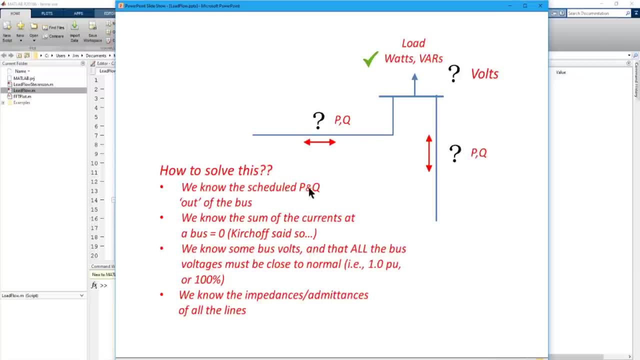 Well, we said before, we know the what's called the schedule, demand or power at this bus. We know the watts and VARs based on a lot of historical data and real time measuring. OK, now we also know what's called Kirchhoff's law. 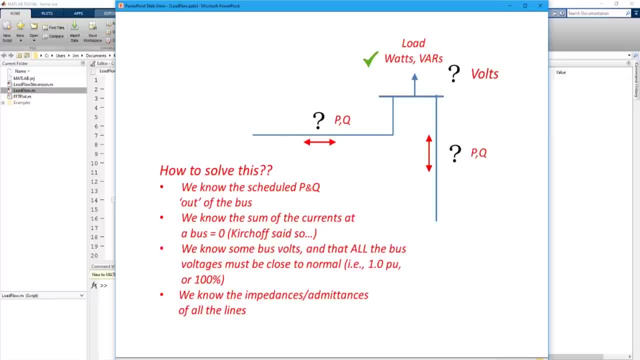 And in engineering you learned that the sum of all of the currents at a normal speed, All of the currents at a node, equals zero. So we know that at this bus, we know that the sum of this current on this transmission line, plus this current on this transmission line, plus this current going to the load, 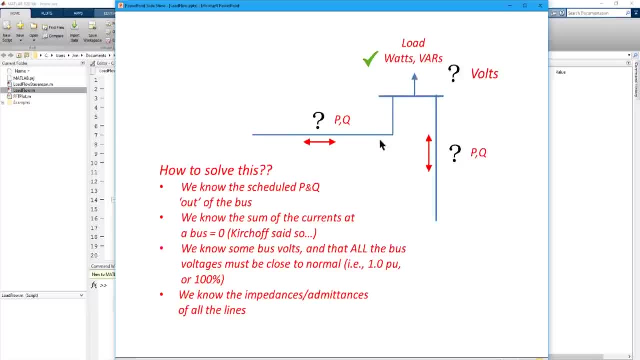 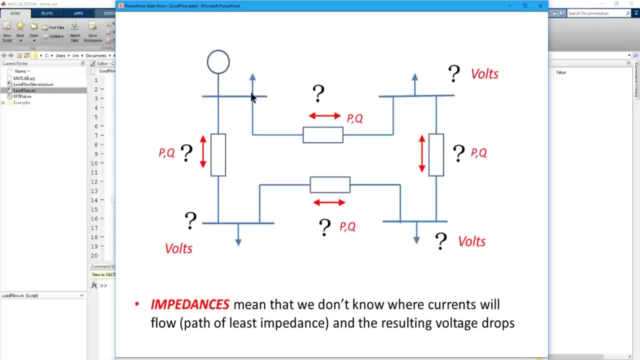 You add those together and you get zero. OK, now we also know, as we mentioned back here, that we know some of the bus voltages. At this generator. it's got a voltage regulator, So we know that what that set point is going to be. 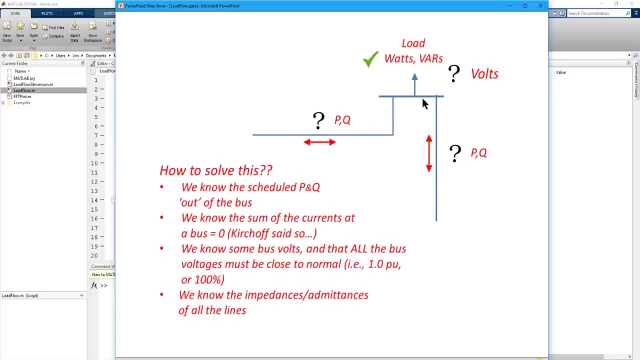 So we know that voltage at that bus. So at some buses we do know the bus voltage because it's fixed with a voltage regulator. In this case, we don't know the bus voltage at this bus because there's no voltage regulator. But the other thing we know is we can give an educated guess about the voltage at the other buses. 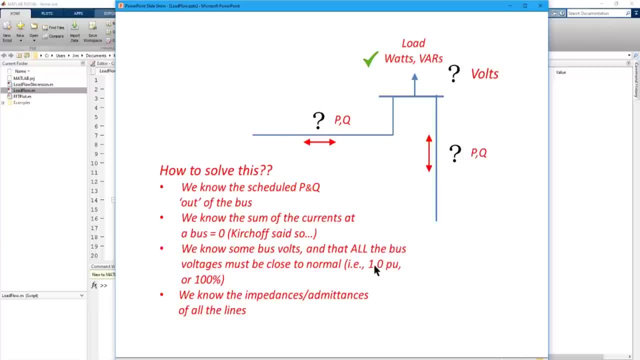 because we know it's all going to be around one per unit, Because we know that it has to be maintained in a strict range, usually around plus or minus 5 percent or maybe 10 percent. So we know that as a guess we can say it's what the voltage is going to be. 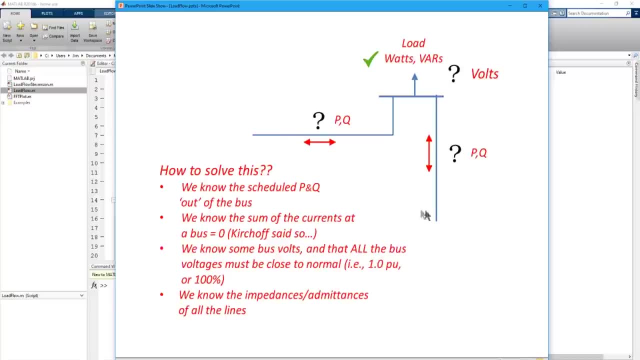 We can make an educated guess. So we may not know it, but at least we can guess it and that might help us. The other thing we know is for each transmission line we know the impedance, or admittance, which is just the inverse of the impedance. 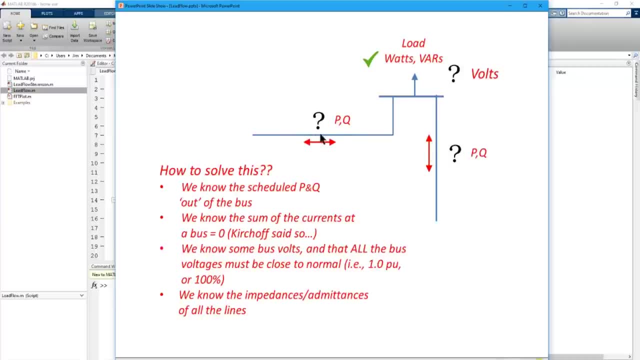 That we can calculate very easily And in fact each transmission line is going to be somewhere around half an ohm for every mile of transmission line And that varies. but that just gives us a ballpark and we can calculate the exact value which utilities do. 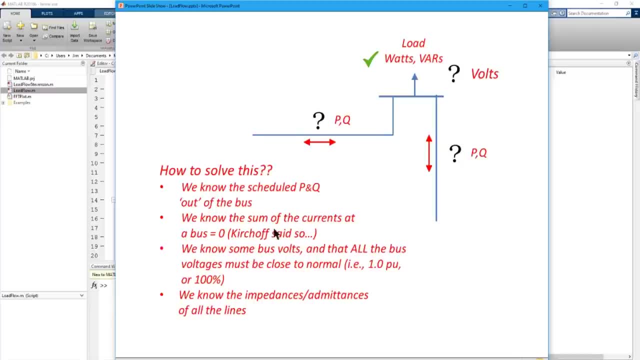 So we know some things. We know the power here, We know Kirchhoff's law, We know some of the bus voltages in the system And we can guess at least a starting estimate for the others. And we know these impedances of all of the network elements. 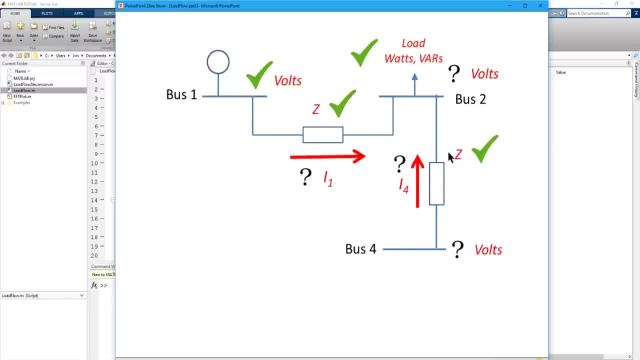 So here's an expanded diagram of what we know. We know the bus voltage at this bus, Bus number one. it's a generator bus. We know the impedance of this line. That's easy to calculate. We know the watts and bars of this load. 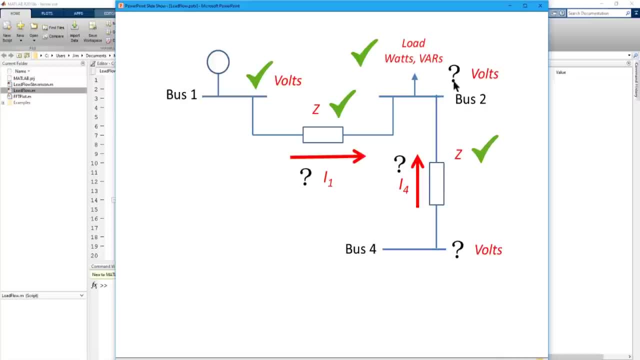 We know the impedance of this line, We can calculate, But what we don't know is the voltage at this bus, Bus number two, The voltage at this bus, number four, And these two current flows on these two lines. Okay, so we know some stuff. 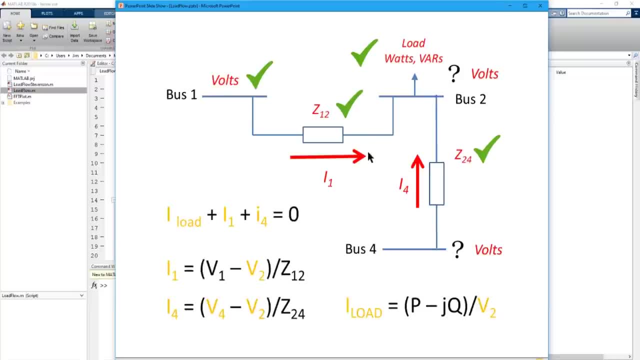 But we still don't know some other stuff. So let's put what we know to work for us and see if we can figure out an answer on these flows and this final bus voltage. Well, we'll take Kirchhoff's current law. 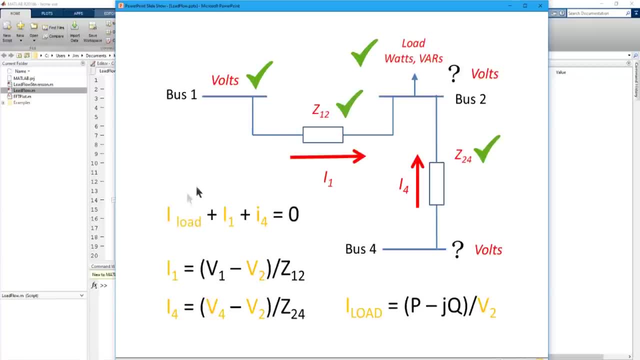 and we'll say I load, which is the current, going to this load, plus I1,, which is the current on this line number one from bus one, plus I4,, which is the current, from bus four to bus two, equals zero. 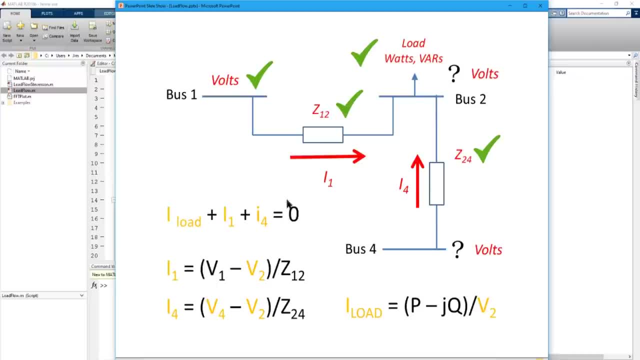 We add them all together and it equals zero. So can we make an equation for I1?? Well, we know that the current through an impedance is basically the voltage across the impedance divided by the impedance. That's basic Ohm's law. 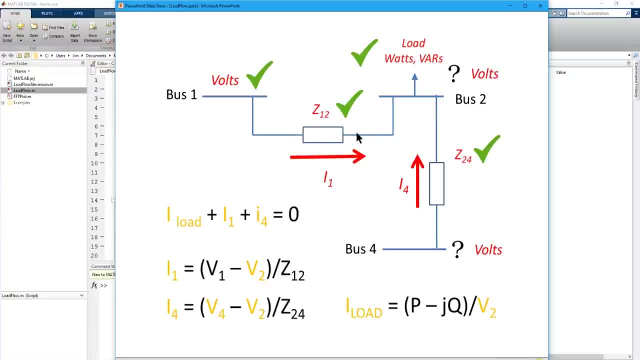 So what is the voltage across this impedance? Well, V1 minus V2 is the voltage across this impedance. So V1 minus V2, divided by Z12, is the current through this transmission line. So down here we've got that equation. 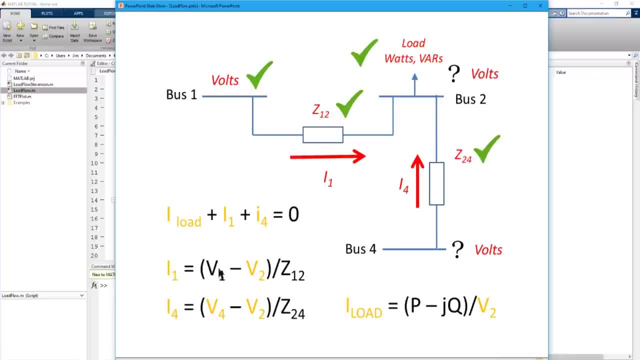 I1 equals V1, which we know it's a fixed voltage, minus V2, which we don't know- divided by Z12, and we know Z12.. Okay, so we've got one equation. now We can do the same thing for this line, from bus four to bus two. 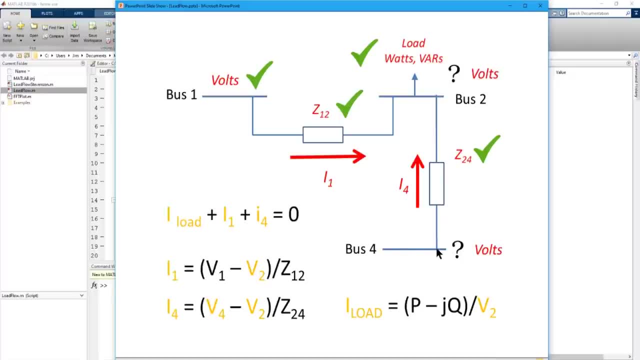 to figure out I4.. I4 equals V4, this remote bus voltage minus V2, the local bus voltage divided by Z24.. Okay, so now we've got two equations for Kirchhoff's law. What's the equation for this current? 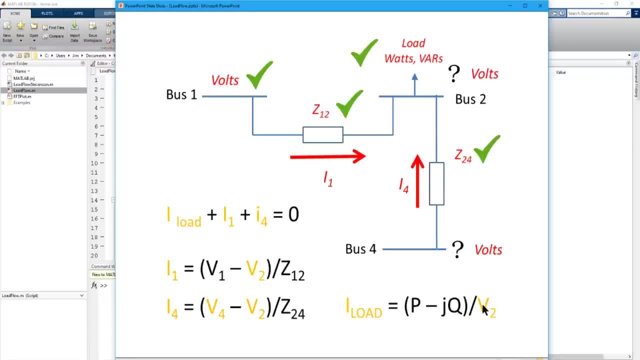 Well, that's pretty straightforward. We know that power equals voltage times amps. So power, which we know P minus JQ, which is the load, watts and Vars, divided by the voltage at the bus, which we don't know, V2,. 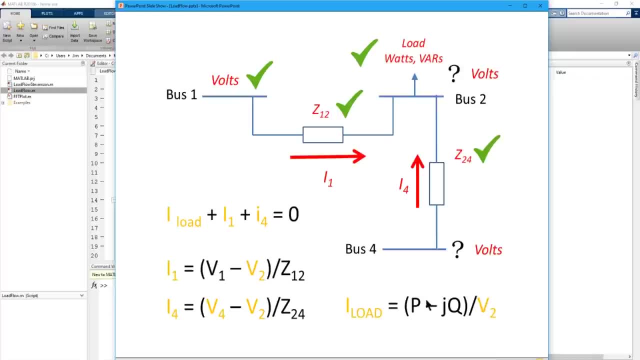 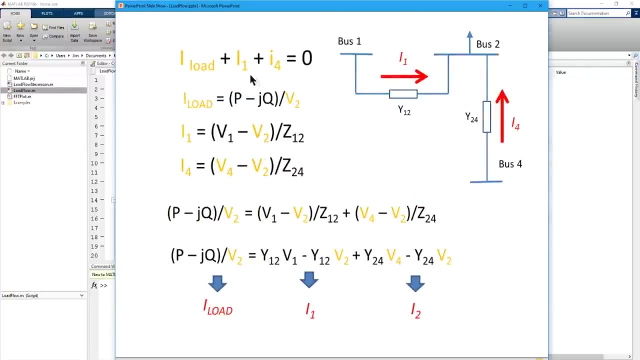 equals the load current at that bus. Okay, very straightforward, just simple calculations to get equations for each of these currents. Now what we can do is plug these into this Kirchhoff's law. And here we've got. we'll just reprint what we had in the last slide. 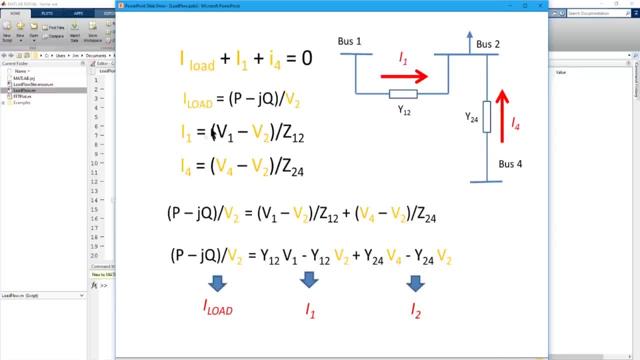 Kirchhoff's law, The formula for the load current, the formula for the current on line one and the formula for current on line four from bus four. Okay, so if we plug these into this Kirchhoff's current law, we will get P minus JQ divided by V2,. 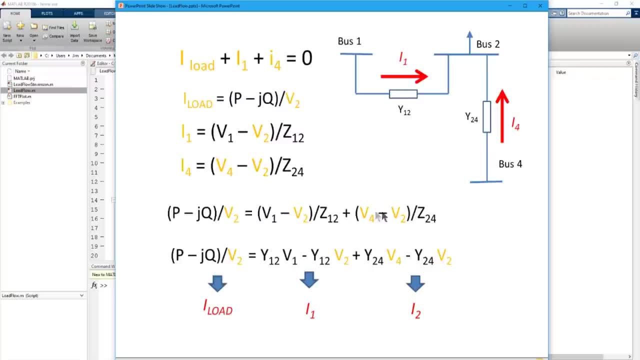 which is just this load. current equals I1 plus I2.. And I1,, like we said, is V1 minus V2 over Z12,, plus V4 minus V2, over Z24.. Okay, very simple. just voltage divided by impedance equals current. 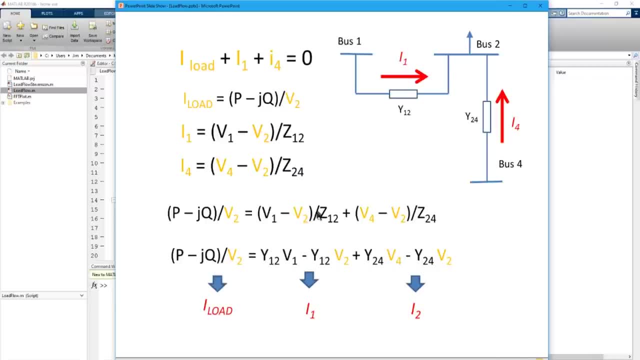 Now what we can do is we can convert these impedances to admittances, And we won't go into detail why we do that, but we'll talk in one of the next videos about why it's easier to work with admittances. 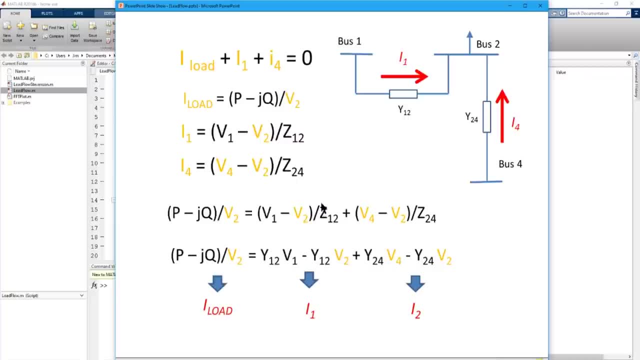 But all we're going to do is we're going to invert this Z12 and convert that to an admittance. So now we've got V1 minus V2 times Y12, plus V4 minus V2 minus Y24.. No change. 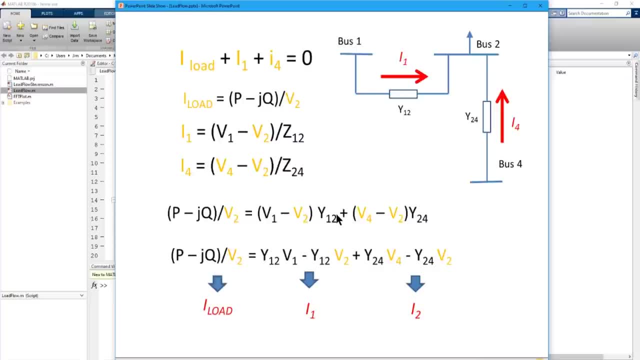 It's just: we're just converting this to admittance and now we multiply, And then what we can do is we can break this out, multiply these out and you will get this equation. Okay, Again, it's just V1 minus V2 times Y12.. 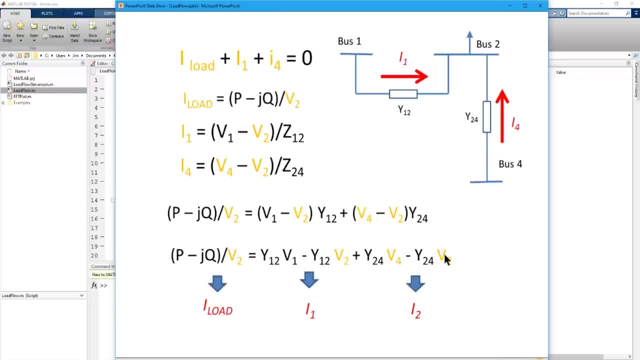 That's I1.. V4 minus V2 times Y24, which is I2.. So all we're doing again is just Kirchhoff's Current Law and we're just putting in this format with voltages and admittances. Okay. 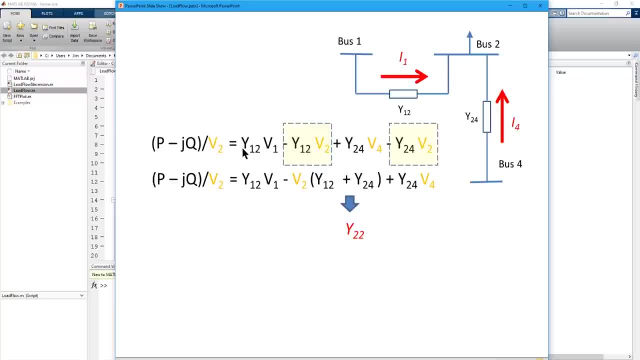 So now, if we look at that equation we just developed- V1 minus V2 times Y12,, V4 minus V2 times Y24, we can see that there are two elements that are multiplied times V2.. Now an important concept to get your head wrapped around here. 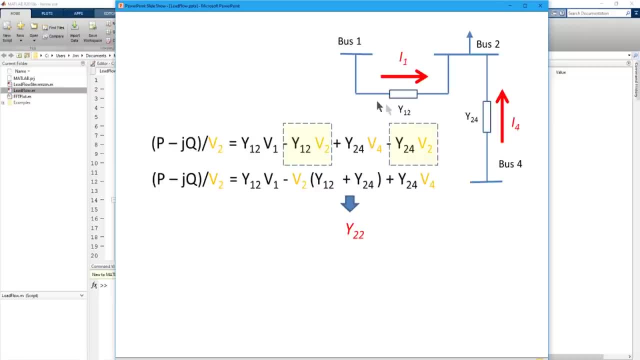 is that you can kind of look at these current calculations on these transmission lines as a remote component, which is, in this case, V1 times Y12, which we've got here, and also a local, what I call a local component, which is V2 times Y12,. 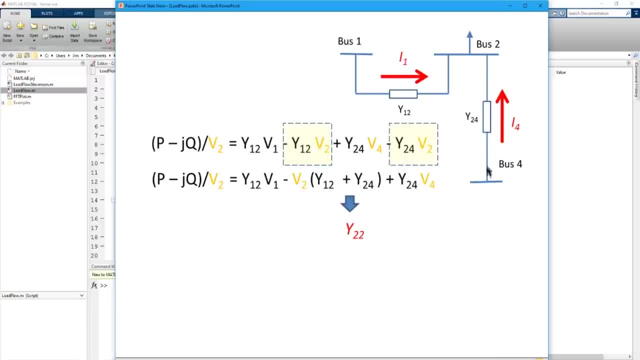 which is this: Okay, Same thing for this transmission line. You've got a remote component- V4 times Y24, and you've got a local component which is V2 times Y24.. Okay, So you can, if you think about it. 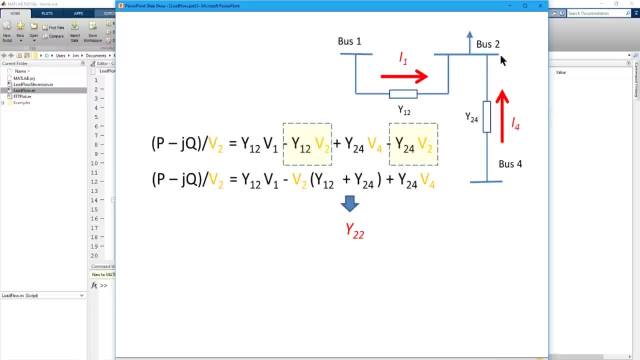 if you keep adding transmission lines here, they're always going to be a remote component. So if we add another bus, say bus 5, it's going to be V5 times Y15, and there's going to be a corresponding local component. 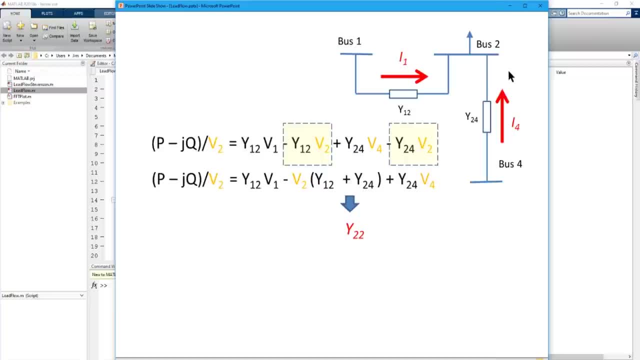 which is V2 times Y15, or Y25, sorry, So we can gather all of these- what I call the local components, together and simplify. So here, what I'm doing is I'm taking this V2 and making a single component. 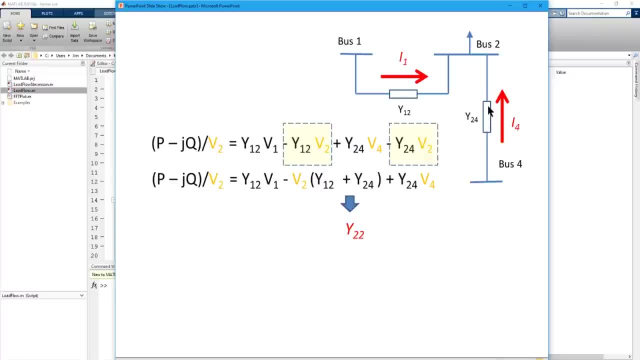 which is the sum of the two admittances of the two transmission lines coming into V2, into bus 2.. So I've basically got Y12 plus Y24 times V2.. So it's this equation, but I'm just bringing the V2 local elements together. 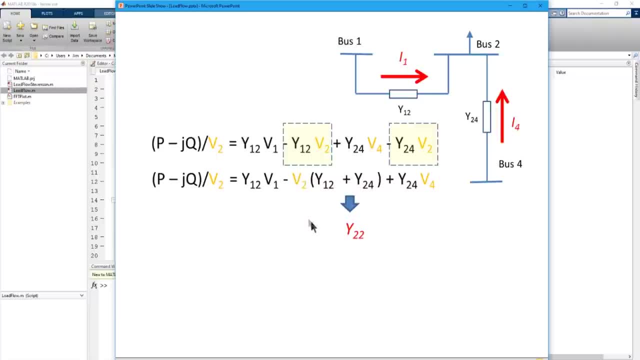 to generate kind of what I call a local component of the current calculations. And that's a very important concept to get in your head, that you've got like a remote component of the current calculation for each of these, for every, basically for every remote bus. 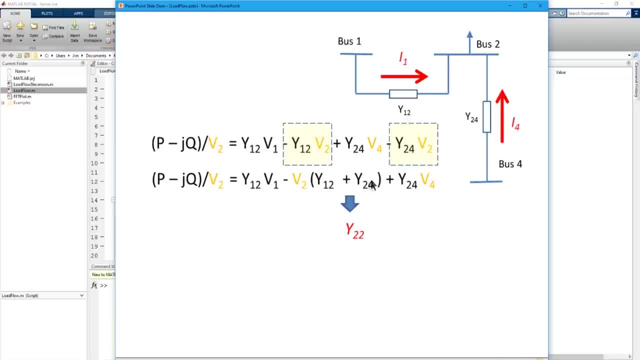 that has a line coming into bus 2. And you've got this local component and we're bringing all the local components together into one package. So for this bus we've got the sum of these two admittances and we're going to bring them together. 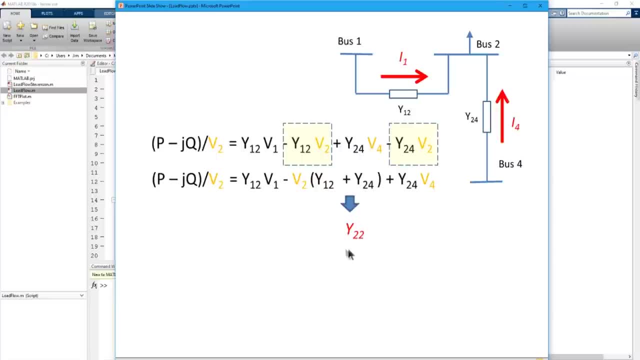 and make one element which we call Y22. And that's just our choice to make this element that we're going to decide to call Y22. And that is what they call a self-admittance, basically the sum of all the admittances. 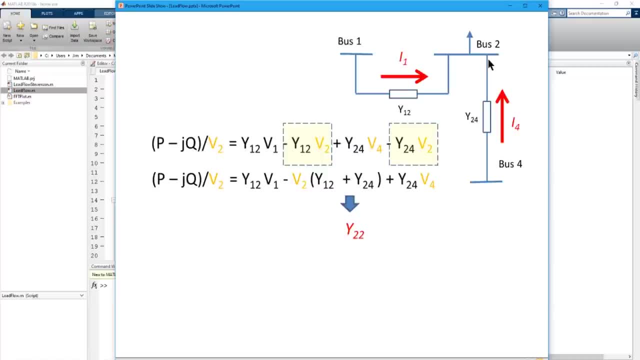 of all the transmission lines coming into the bus that you're solving for. Okay, Again, a very important concept that we have this self-admittance of the bus and again it's just basically the local component, the package of all the local components. 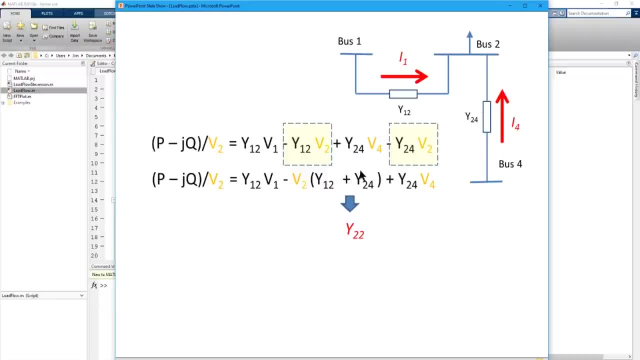 of the current calculations for all of the lines. Okay, Again, a very important concept to get your head around. So, now that we've got this, we've replaced these by a Y22, the sum of the admittances. here's the equation that we're going to try and solve. 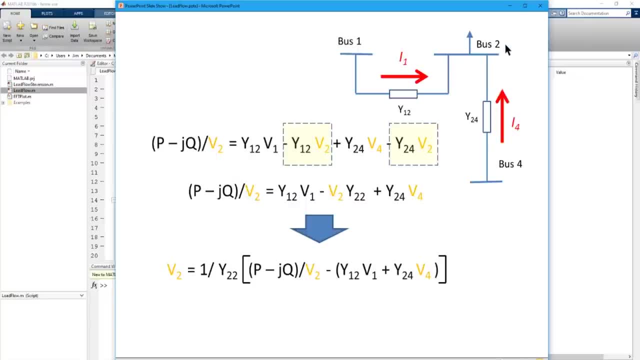 and see if there's some way we can get a solution for the V2, the voltage at bus 2.. So here's our equation, our simplified equation, and what we want to do is: let's see if we can take this V2 here. 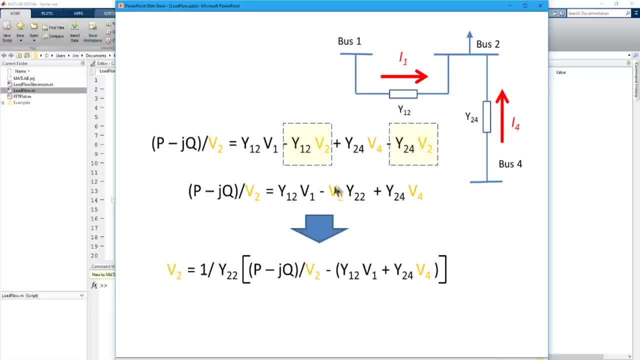 and see if we can pull this out and put it over on the left-hand side of the equation and then shift everything over to the right-hand side. So it will be: V2 equals all the other stuff. So we're just pulling this over. 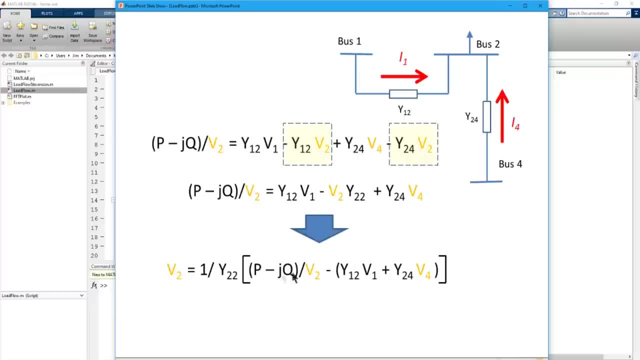 If we do, we come out with this equation down here. It's basically this equation, with this one V2 moved over to the other side, just rearranged, And it's basically: V2 equals 1 over Y22,. okay, because we're going to pull this over. 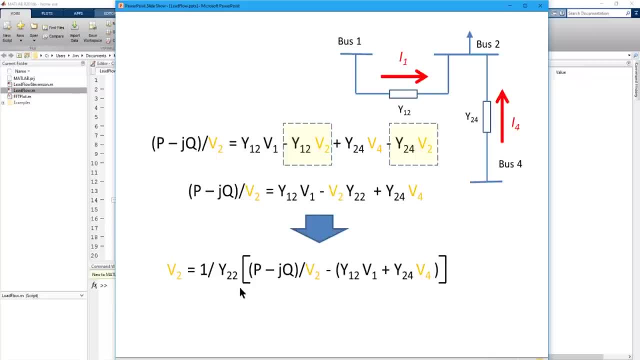 so we've got this Y22.. We're going to multiply the rest of the equation by times your I2 component, the current based on the load at bus 2, plus the remote components of the line. impedance calculation: Okay, V1 times Y12,. 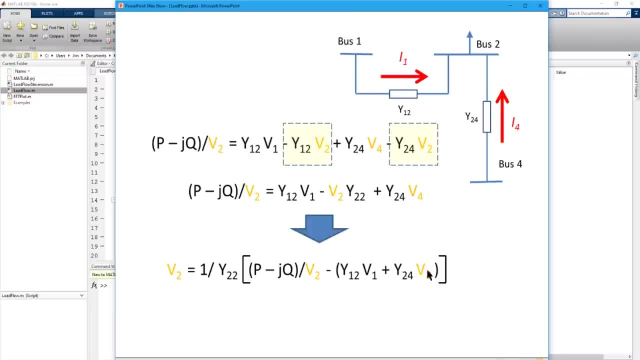 which is the remote component, plus V4 times Y24,, which is the remote component of the current. Okay, so that's all we're saying. This is the V2 we want to solve for, and it's basically just the equation we've been working with. 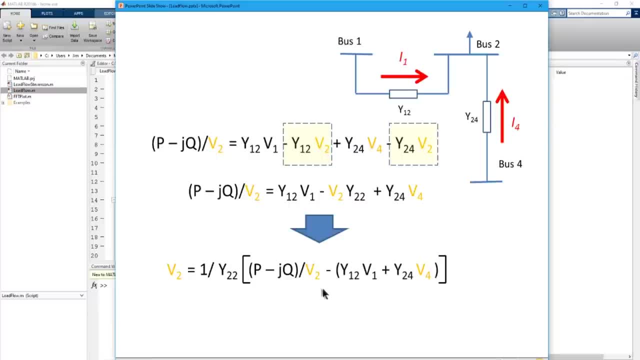 Now, if you look at this, you say wait, wait, wait. How are you going to solve for V2 if you've got a V2 in here and you don't know the answer. You don't know what V2 is. 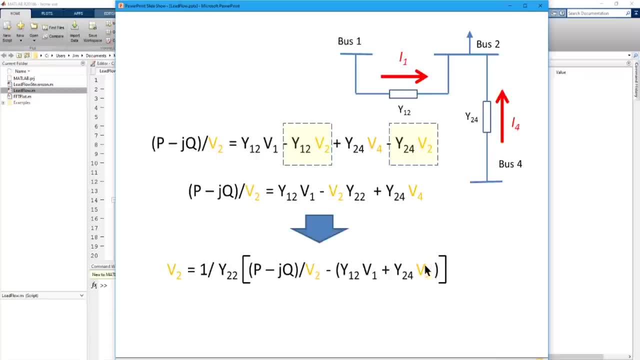 and you've got a V4.. You've got two unknowns here: V4, you don't know what V4 is and you don't know what V2 is. How are you going to solve that? Well, that brings us to another very important question. 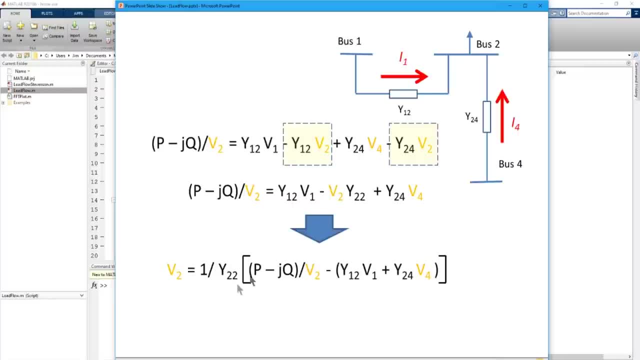 It's a concept you need to wrap your head around when it comes to solving these networks, and that is the concept of guessing and iterating. Okay, so what we're going to do is we're going to guess the unknowns and use that to iterate. 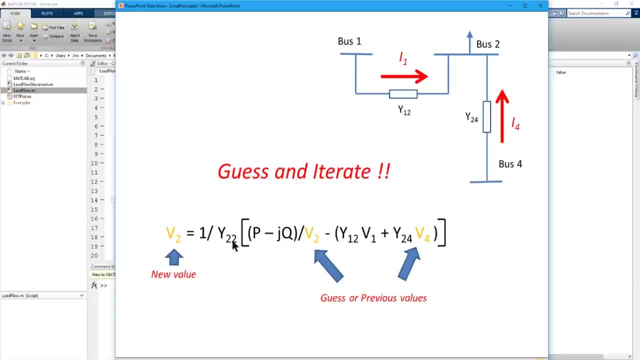 and let me give you an example of how we're going to do that. Here's our equation for V2, and we've got these two unknowns. What we're going to do is we're going to guess at values for these two. 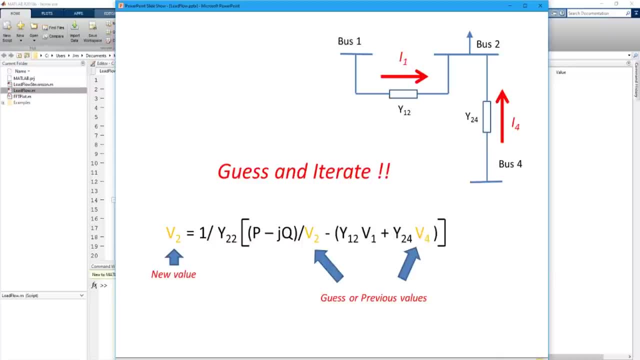 and, like I said, we kind of sort of know what the value is going to be. It's going to be somewhere around one per unit. So we can just put numbers in these two values, solve the equation and that will give us a better value for V2.. 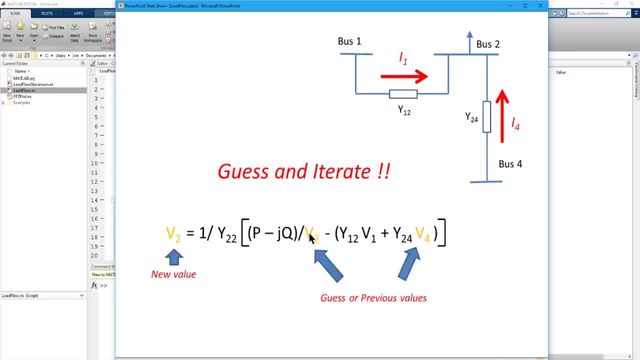 It's not going to be the final value, but it will be at least a starting value that we can use for V2.. Now, once we've got that, what we can do is we can take that new value for V2 and put it back into this. 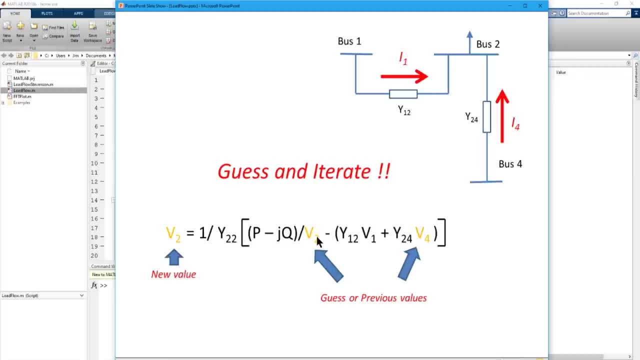 replace the old value- the initial guess- with this new value and re-solve, and that will give us an updated V2, and it's going to be better than the old one. It's not going to be the final answer. 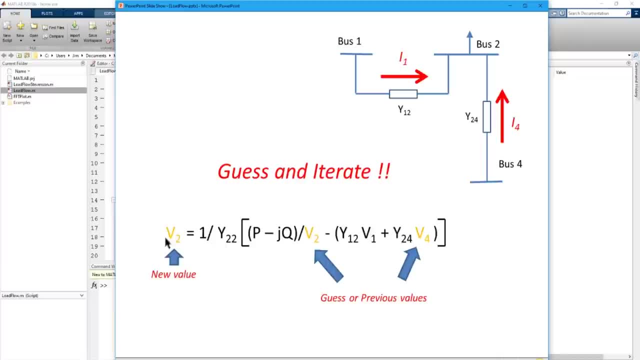 but it will be better than the old one. Now, keep in mind we can keep doing this and doing this and, if all goes well, that V2 is going to converge to a final value and it's going to stop changing as we keep iterating through. 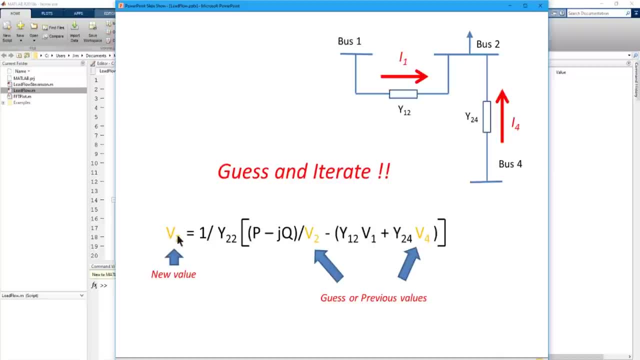 hopefully it will converge to a final value. Now, is that the final correct value? Well, no, because throughout this we've been using this V4, which was just a guess. Okay, So we can get a better V2,. 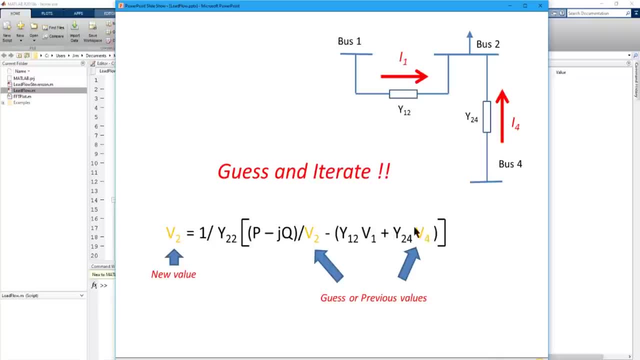 but we can't get the final V2 until we get the final V4, which means we're going to have to iterate around the system and do this same procedure throughout the system until everybody agrees we've got the final value, And we'll talk about that a bit in the next video. 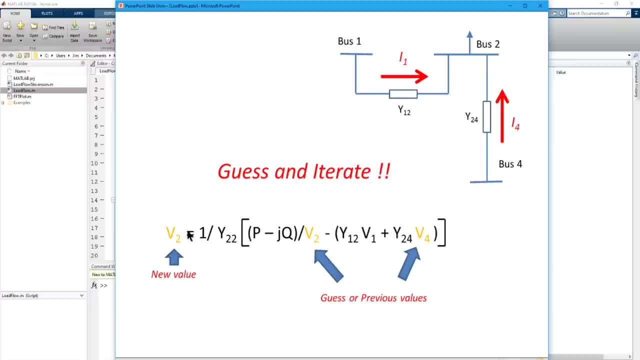 but what I want to talk about now is I want to show you a visual example of how this works, how we can start with a guess and iterate through a few times to get an improved value for V2 on this bus and each time see how it's starting. 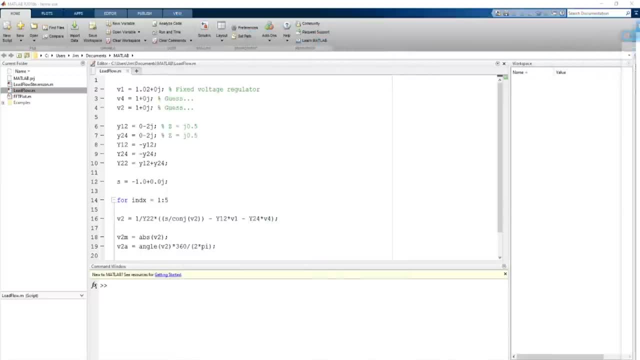 to converge to a final value. Now the way we're going to do that is we're going to fire up MATLAB, but we haven't used MATLAB. MATLAB is a very useful. what I consider is kind of like a super calculator where you can do real-time interactive. 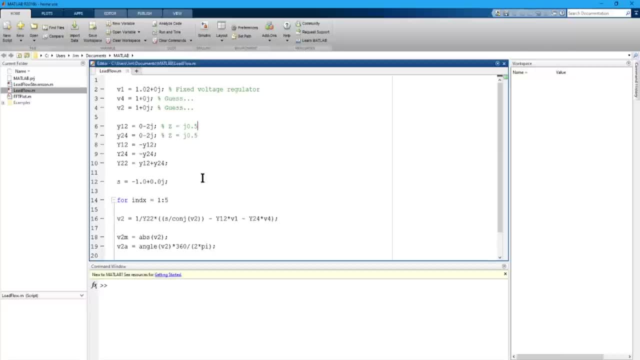 solving of equations and you can graph them and you can do a lot of real-time analysis. And what's nice about MATLAB is it works. it's based around matrices. So if you're going to do stuff like these network calculations- 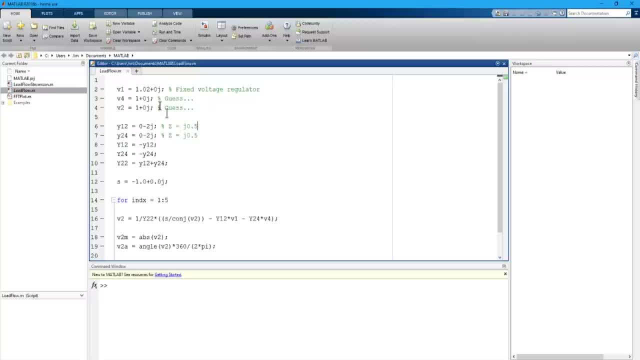 you can do matrices and you can do complex numbers. We're going to be doing a lot of complex numbers when we're dealing with power system analysis, because all of the impedances and the voltages and the currents and the powers are all complex numbers because you've got watts and bars. 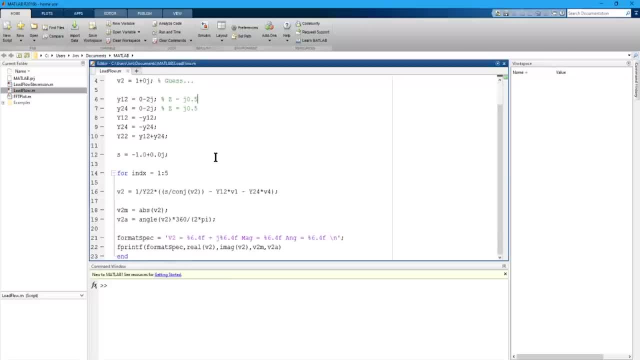 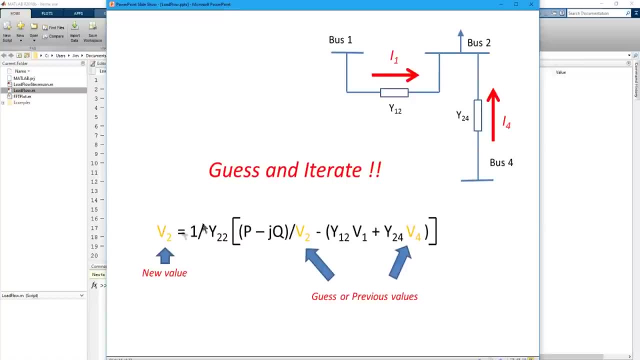 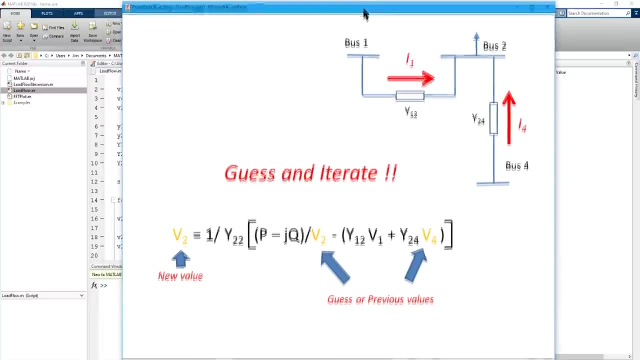 and Rs and Xs and capacitors. So MATLAB is going to be very useful, and what we're going to do here is we are going to solve this equation just at bus 2, and we're going to iterate through and see how we start to converge. 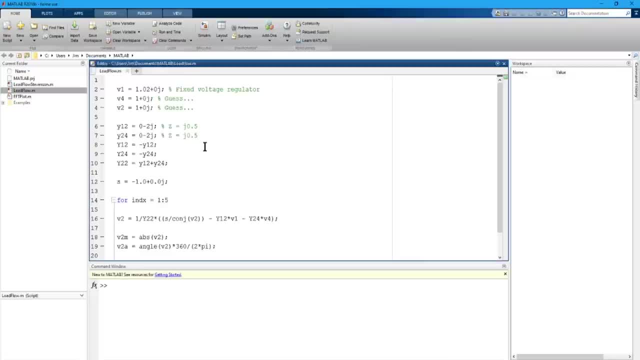 at a better number for V2.. Now here's our MATLAB and what I've done is I've entered previously some commands. I've got about 20 lines of code here and it's fairly simple. I'm just in the first. 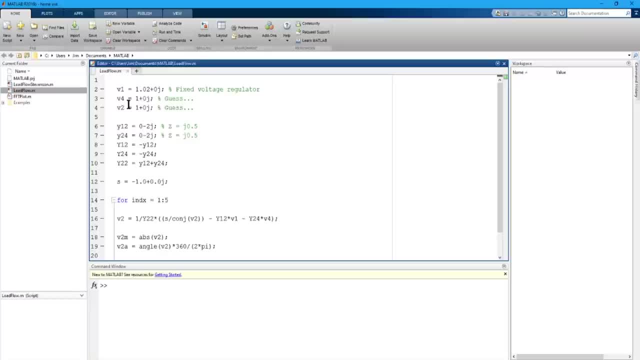 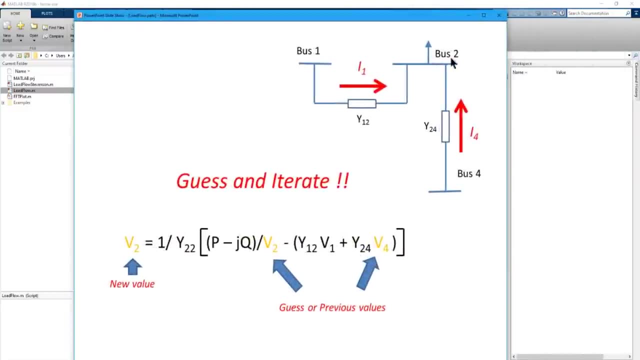 this first three lines here. I'm just starting out to initialize the voltages at the three buses. okay, I've got bus 1,, bus 2, and bus 4, and we said bus 1 is the generating bus, so there's going to be a fixed voltage here. 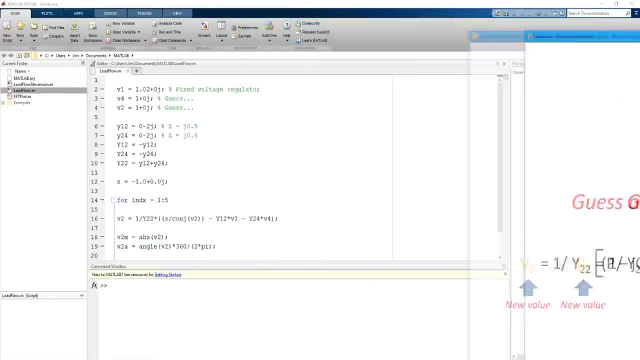 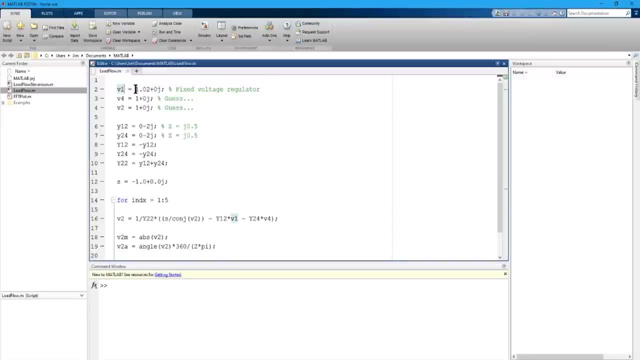 Bus 2 and bus 4, we don't know, but we're going to guess that they're about one per unit. So V1, we're going to say it's a fixed voltage for the voltage regular at 1.02 per unit at an angle of zero. 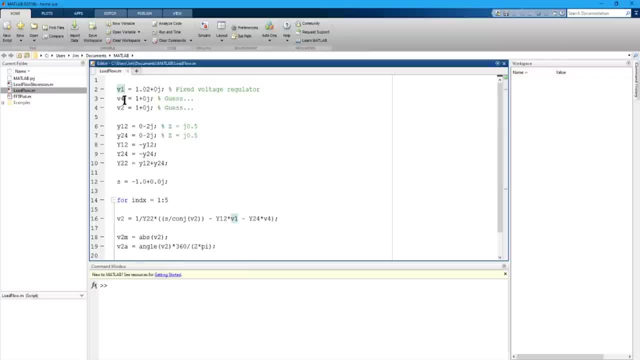 so there's no J component. V4, we're going to initialize it. We're going to start with a guess that it's one per unit normal voltage at zero angle. There's no J component, So here we're just setting up V1,, V4, and V2. 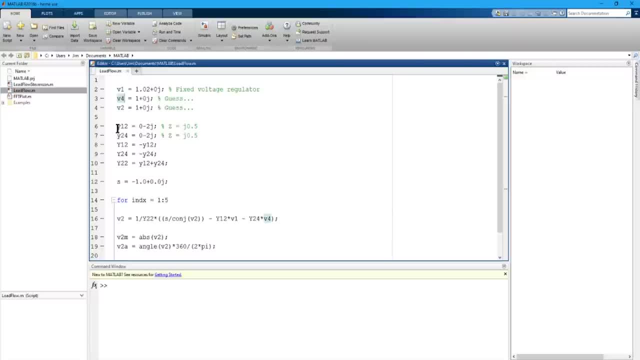 with our guesses and our fixed value. Now, here in 6 through 10, we are setting up our line admittances For the two lines Z12 and Z24, these two values we're going to say they're the same impedance. 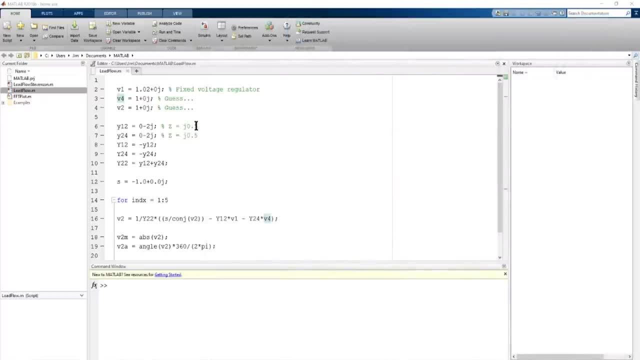 and the impedance value we're going to say is J.5,. okay, So it's a reactance of 0.5 per unit, which means the admittance of that line is 1 over that, which is minus 2J. 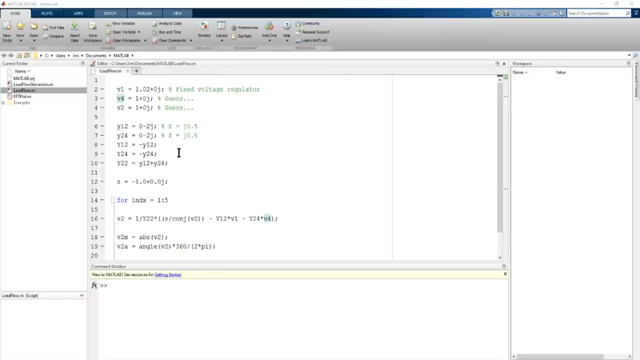 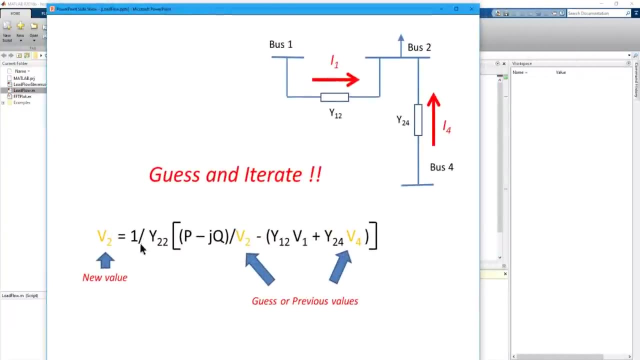 and that's going to be the same for both. Now here we said that we also are going to have a self-admittance. this Y22 value at this bus is going to be the sum of the two admittances. 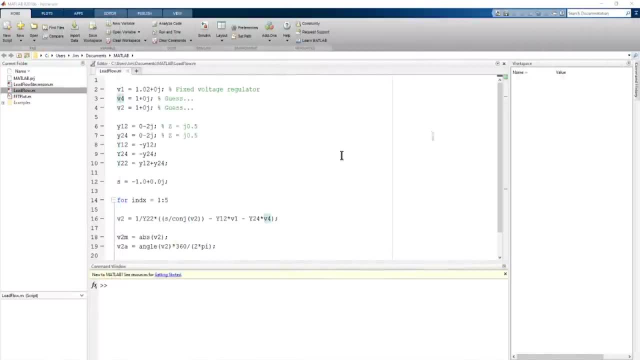 in this case, of these two lines. So here I'm calculating: Y22 is the sum of Y12 plus Y24.. Now the last thing we're going to initialize is this: power at bus 2, and we're going to say that the power is. 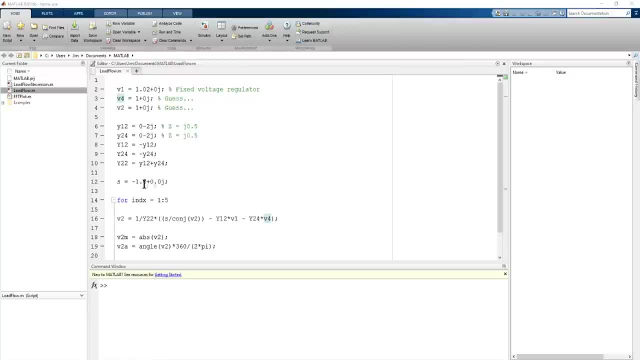 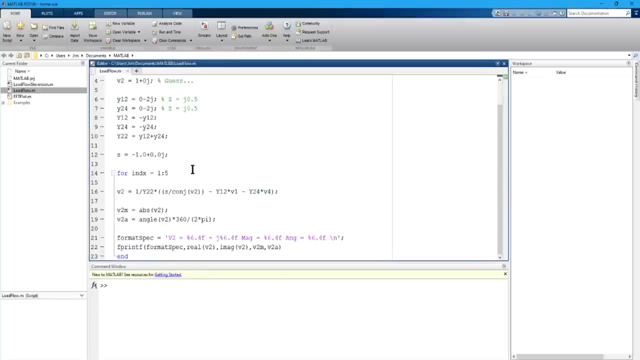 minus 1 per unit watts and 0 Vars. So minus 1 because it's out of the bus, it's going to the load and no Vars. okay, So now we've initialized everything and what we're going to do in this for loop. 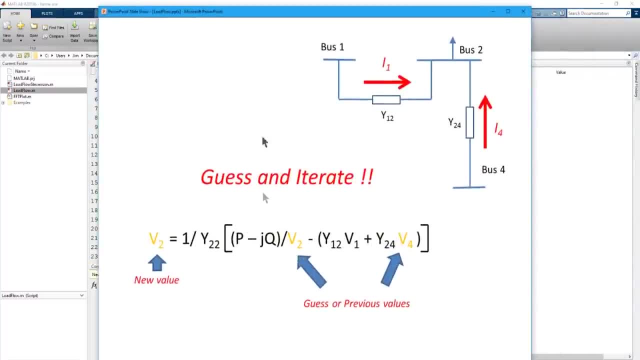 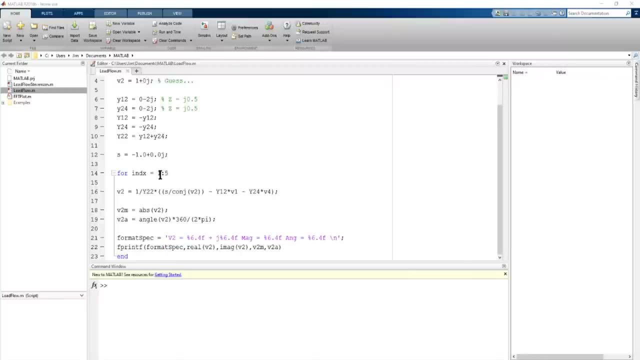 is just solve this single equation right here that we did before and we're going to iterate through 5 times. So for the index is 1 to 5 between this 4 and this end loop, and we're going to iterate 5 times. 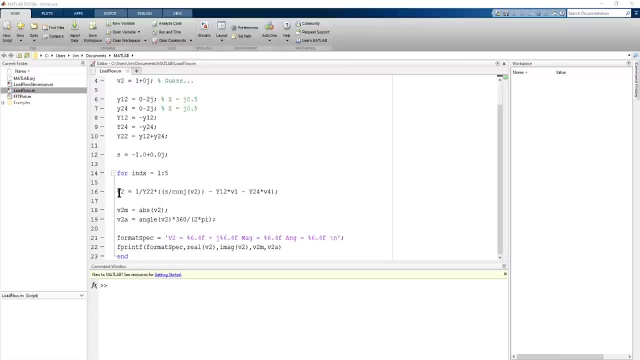 and just solve this equation. And the equation is: V2,, like we said before, equals 1 over Y22 times S, which is the power divided by V2, and we're using the conjugate we'll discuss later- minus Y12 times V1,. 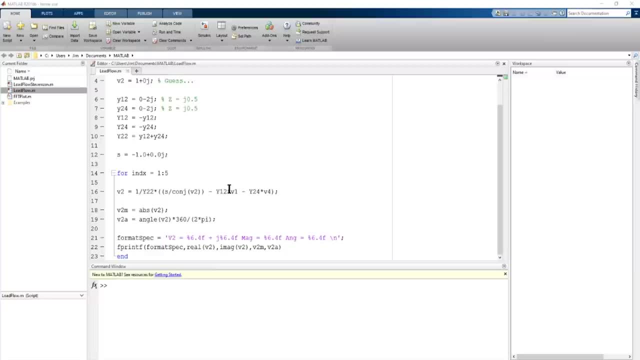 basically the remote component of the current from bus 1, minus the remote component of the current from bus 4,. okay, So we're going to start out V2, and it's going to use this initial guess of V2, and it's going to use the fixed value of V1. 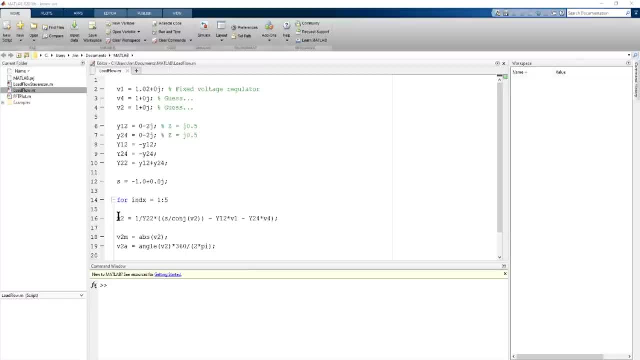 and the initial guess of V4, and it's going to calculate a new V2.. And here I'm just calculating the magnitude and angle of V2 that I'm going to print out. and here's just the printout, so you don't have to worry about these. 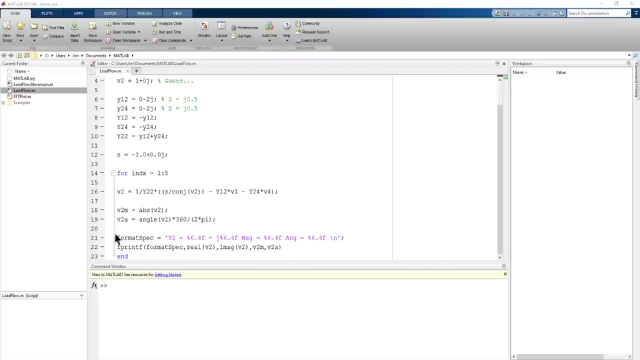 but I'm just going to go 5 times and it's going to calculate V2, and next time it's going to come in and use the old value of V2, with the initial estimates of V4 and V1, and it's going to calculate a new V2. 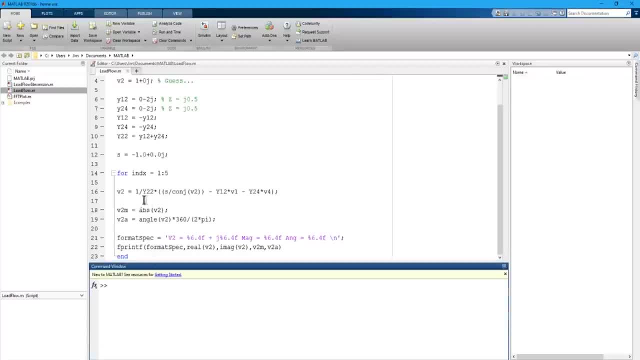 and print that out. So basically what I'm going to do is I'm just going to run through this script is called load flow, so I'm just going to run this script and each iteration you can see I've printed out here. 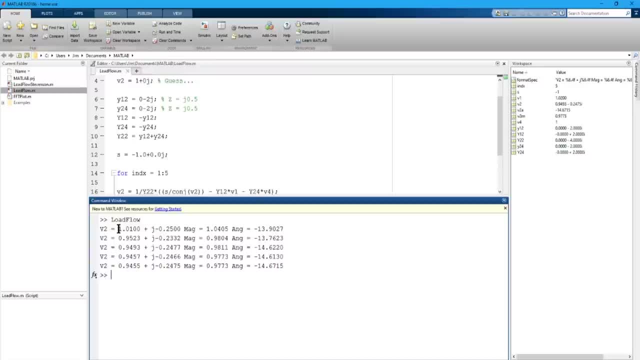 the values of V2, and iteration 1,. the value is 1.01 minus J.2, minus J.25, and that comes out to a magnitude of 1.04 per unit at an angle of minus 13.9.. 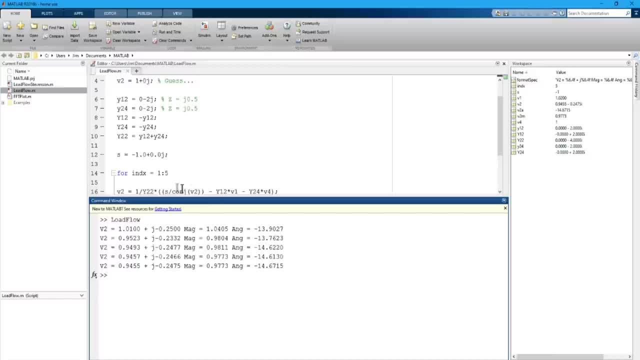 So then it takes that value of V2, plugs it back into this equation and calculates again, And the second time it comes out with: okay, now it's 0.9523 minus J.2332,, which is a magnitude of 0.98. 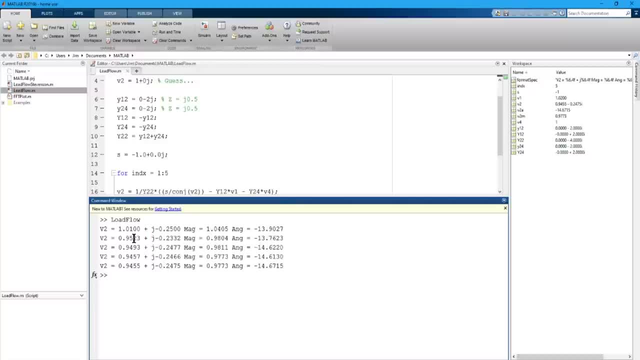 at an angle of minus 13.7.. So you can see it's changing a bit and you get, third iteration, 0.9493 minus J.2477,, which is a value of 0.9811 at minus 14.6.. 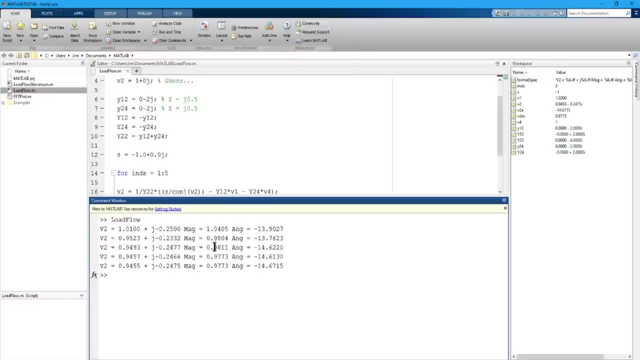 So you see, it's starting to get converge down to 0.98 at an angle of 14.6.. And again we do it. again we get 0.977 minus 14.6, 0.977 minus 14.6.. 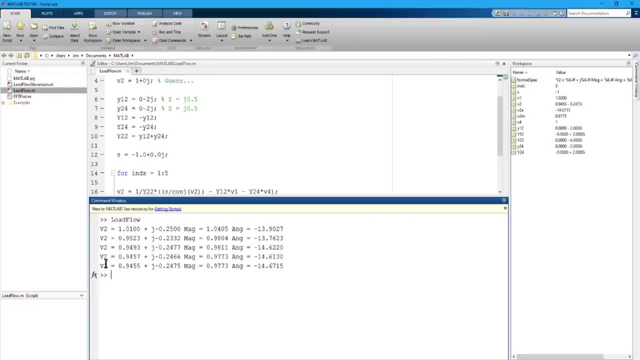 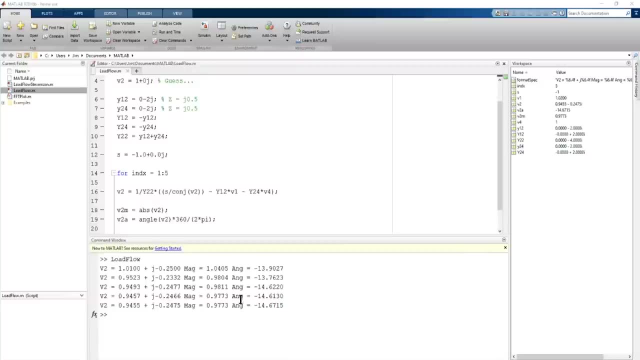 So you can see, after about five iterations, V2 is getting down to be about 0.977, at minus 14.6.. Now, keep in mind, this is not the ultimate correct value of V2. Because, remember, we are using a guess for V4. 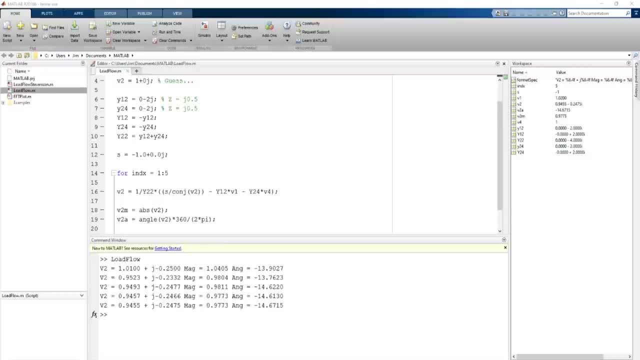 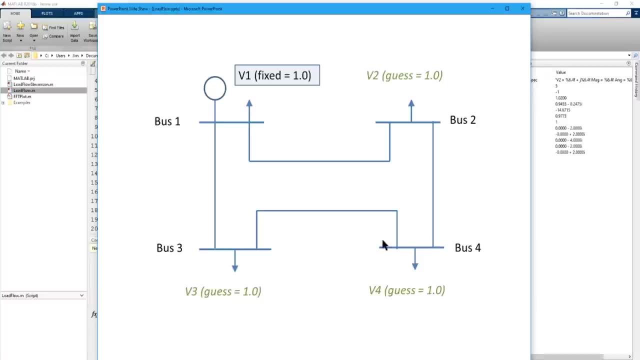 in this equation. So now what we have to do is we have to use our new value of V2 and go throughout the system and get good values for all of the buses. So for example, we started out here. we got our V1 fixed at 1.0 per unit. 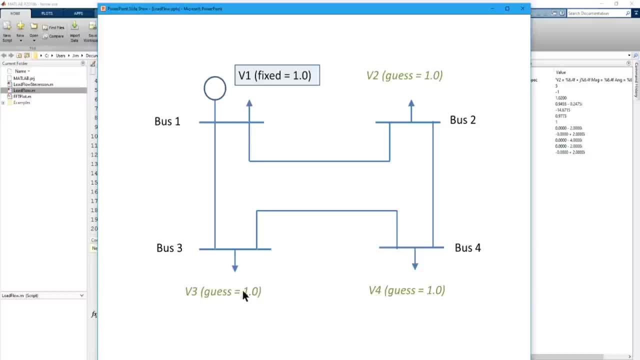 we used guesses for V2,, V4, and V3.. So what we're going to do, we just went through and we calculated V2,, revision 1, say it's 1.02.. So once we've got that, 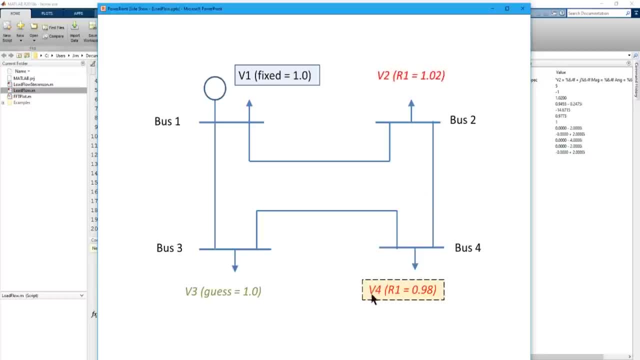 then we're going to go to say bus 4, use that 1.02 from V2 in the equation for bus 4, calculate revision 1 of the V4 voltage. let's say that's 0.98.. Then now we've got these two. 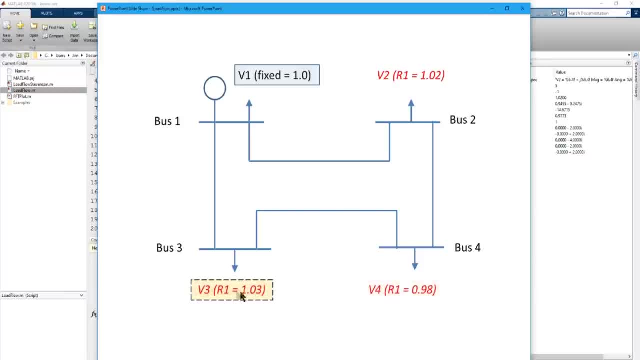 updated voltages for V2, and V4,. we can go to bus 3, and that will give us a revision 1 voltage for bus 3, say it's 1.03.. Now we use these three voltages, go back to bus 2. 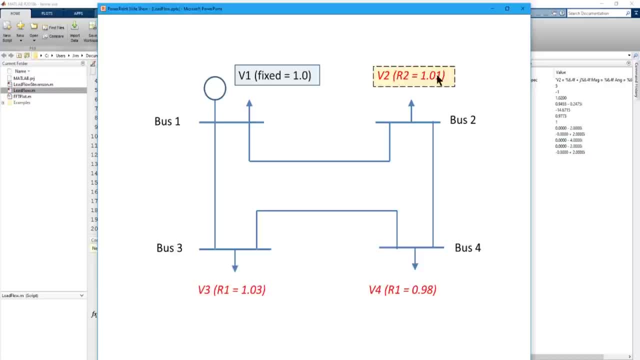 and get revision 2 of bus 2, might be 1.01.. So you can see, we just keep going around the system, updating using our best estimates from the previous calculations of the other buses and at some point we're going to get a final value. 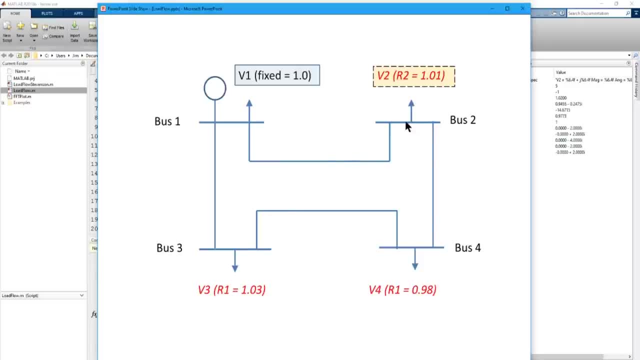 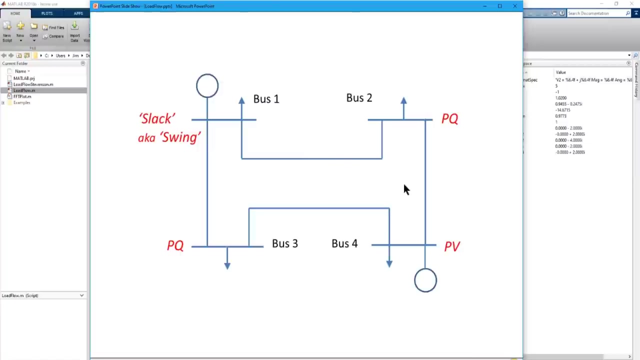 for all of the buses that agree and are within our tolerance. The change between each iteration is small enough that we accept it as the final solution. Now, in some of our next videos, we're going to talk about some of the additional factors to consider. 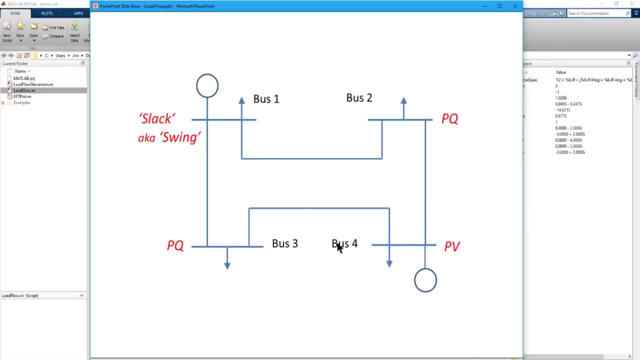 For example, let's say our system here had a generator at bus 4, in which we are specifying the output power and the regulated voltage at the bus. At this bus you need to make an additional calculation for VARs, and we'll talk about that. 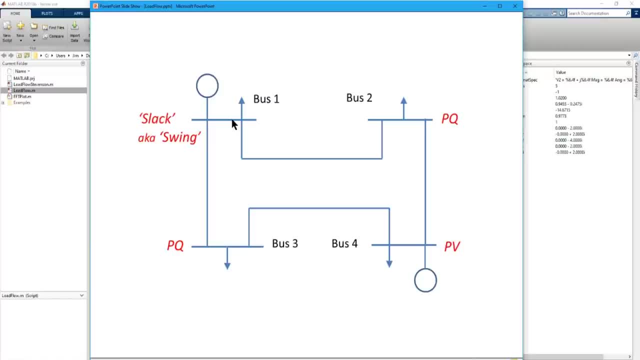 And then there is another bus, generally in a load flow study, that serves to act as what's called a slack bus, also known as a swing bus, and it basically takes up the slack for all of the losses, all of the watt and VAR. 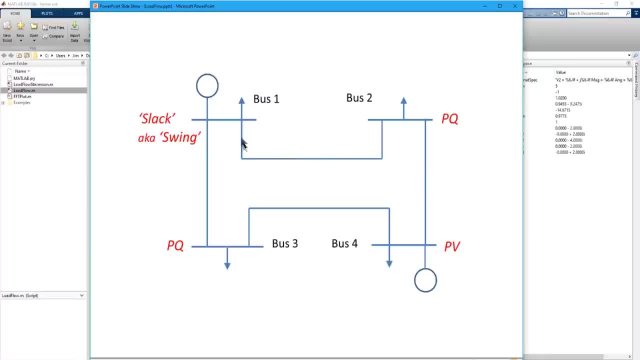 losses in the system It accounts for. as you calculate all these flows and you dissipate watts and VARs in the elements, some generator has to account for those losses and those are all assigned to the slack or swing bus. There are some additional calculations. 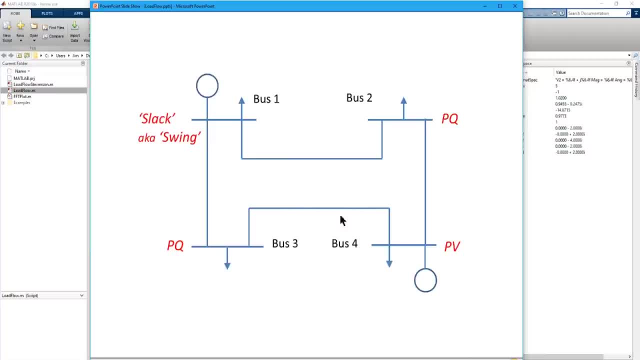 you need to do when doing this, but hopefully you've got a fairly good idea, a basic conceptual understanding on how we do this analysis. In the next videos we'll go through and look at some of the details on how we actually would solve this system based on these. 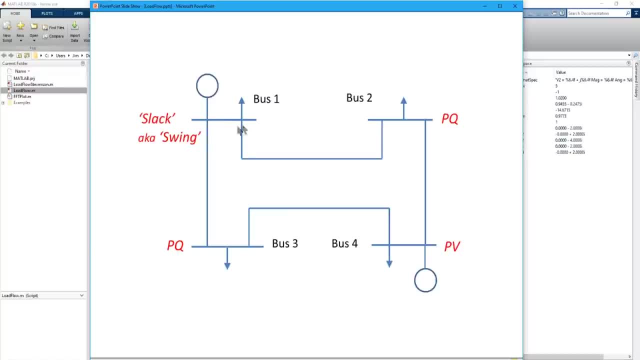 additional types of buses and loads. I hope this has been helpful. Take care and have a really good day.